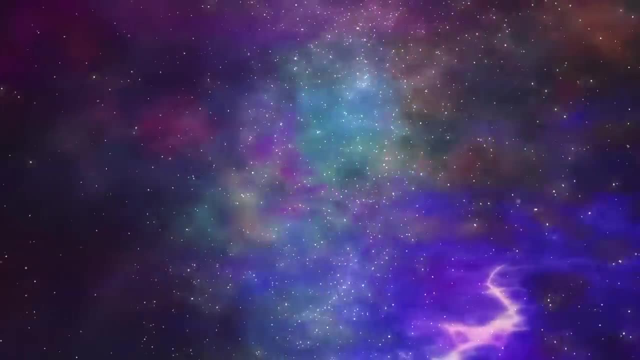 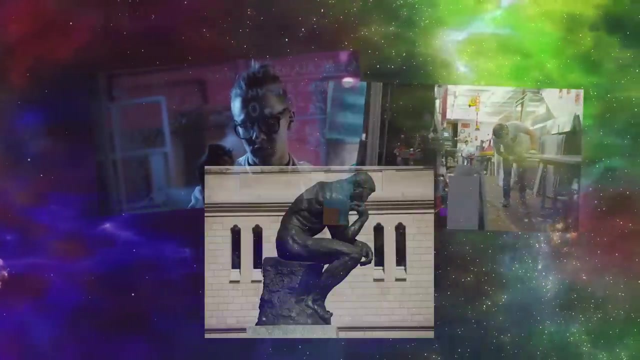 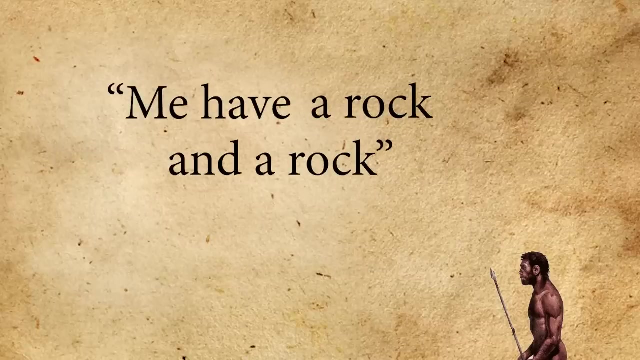 a good moose. Then something revolutionary happens, Something so mind blowing that it changed the world forever. a spiral which has created science, engineering and logic itself. Grook picked up another rock, But instead of saying me, have a rock and a rock. 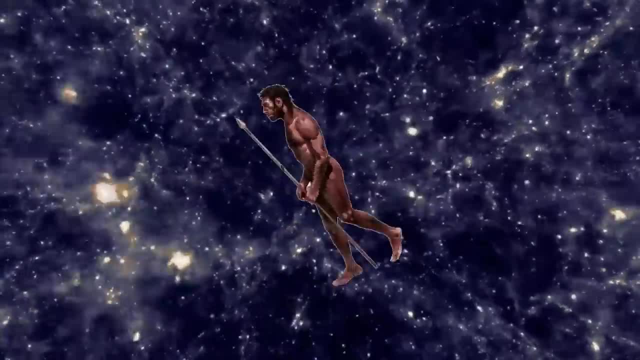 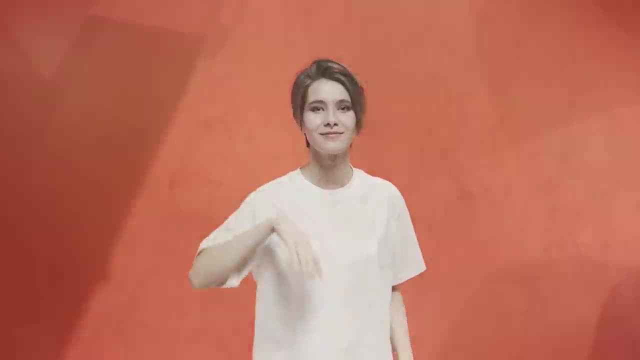 Grook says me, have two rock. And just like that, Grook unleashed the beast of number theory and mathematics itself. Early humans used their fingers to count. One apple means one finger up, two apples means two fingers up. Did I really have to explain it to you? 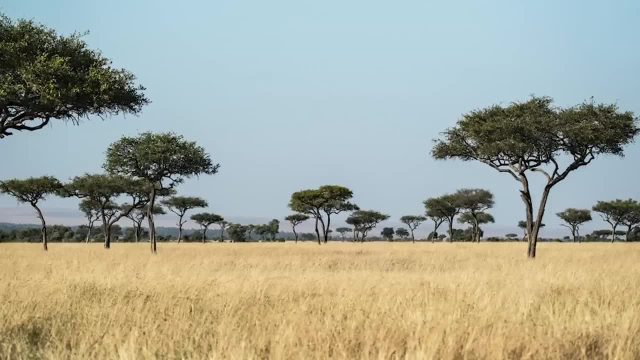 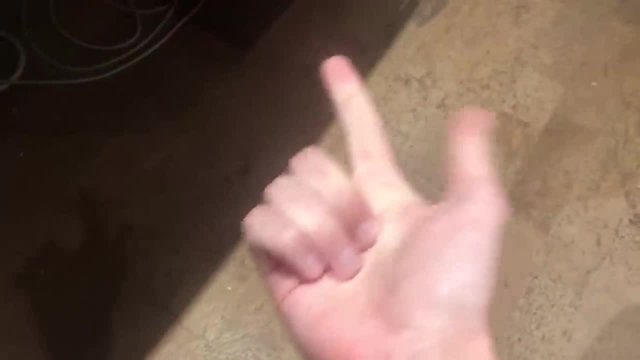 It's likely that counting was the first sign language ever invented, which is a big loss to all the deaf cavemen out there. They could only count at each other. That's good up to 10,. ok, I lied, it's actually good up to 1024 numbers. but come on, you know it's 10.. And humans are big boys now and need 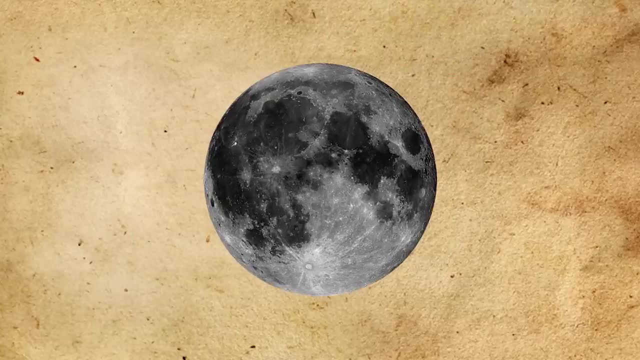 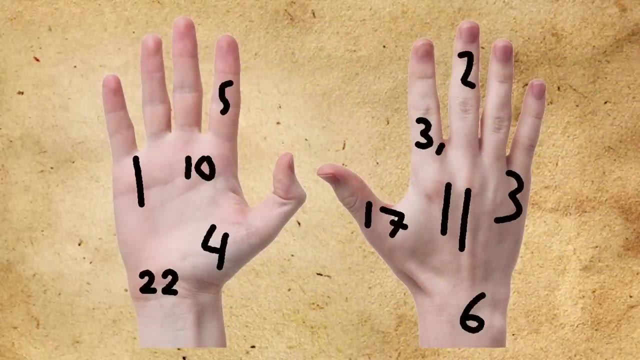 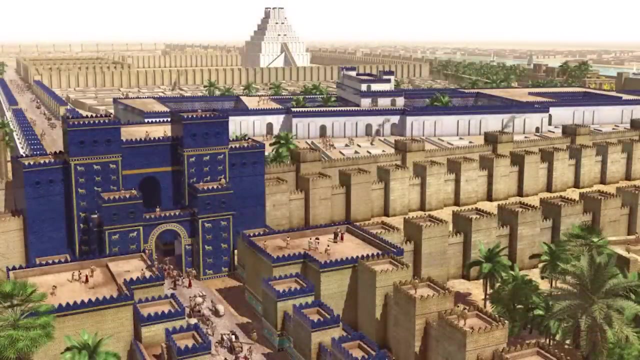 to count, um, I don't know, the moon I guess, Which happens to be in cycles of 30 days. I have an idea: let's put numbers under our hands, or at least under animals' hands. Tally's were counted on bones 40,000 years before writing was ever invented. It's negative. 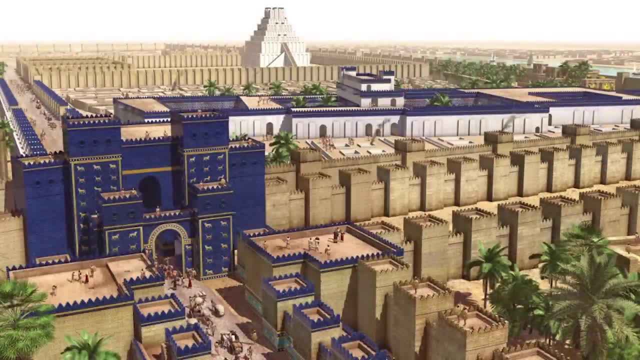 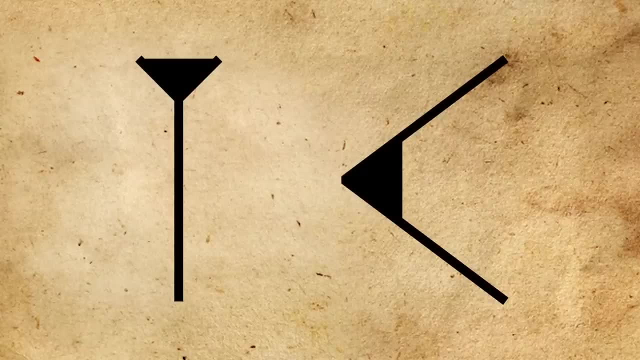 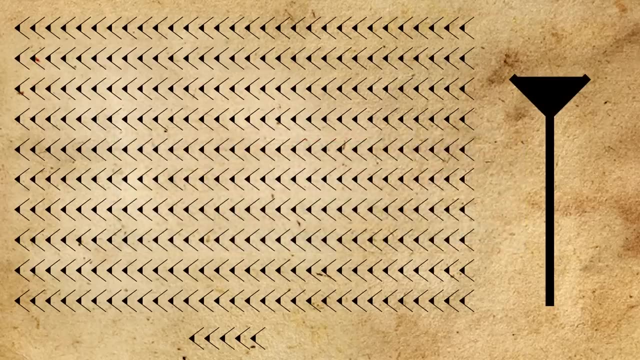 4,000 now. Society was built, clay was harvested and the Babylonians made these things. What a mess. They could only count ones and tens way faster than on hands. but I mean ask them to write down: you know 3051.. Yeah, nice, try guys. At least they kickstarted writing. 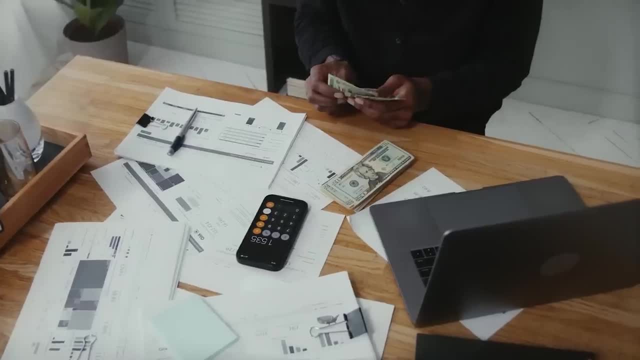 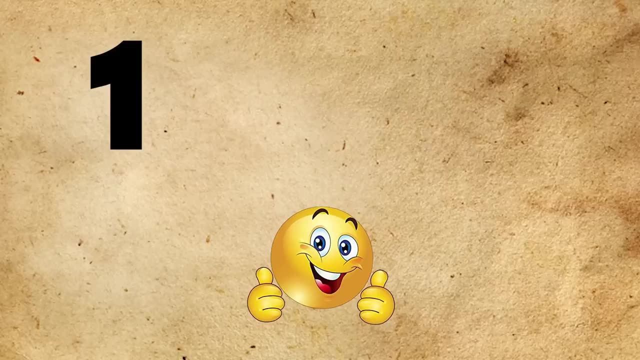 from all their accounting nerd purposes. That's right, all you number crunchers you made writing. Ok, enough fun, get back to my taxes. One is good and two is good, but one and a half. What are you talking about? Around the same time, the ancient Egyptians realized you couldn't. 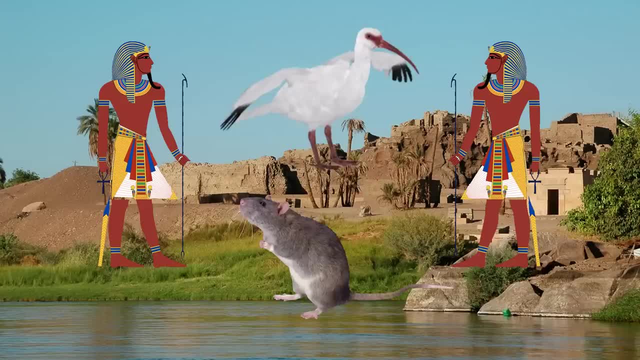 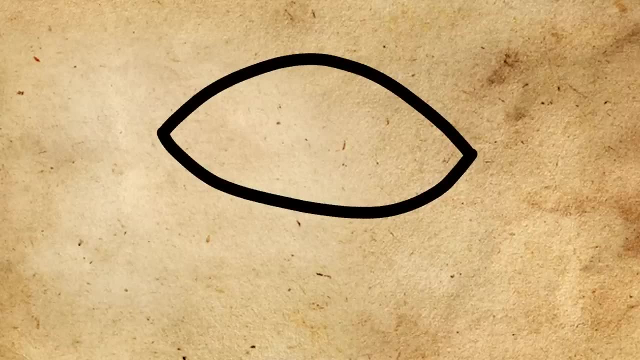 give one pie to two people, or actually a bird or a rat or something. They had an even better way to write numbers, but still awful. What am I looking at? They used this symbol for putting a number on the bottom and only used whole reciprocals, except for two thirds. 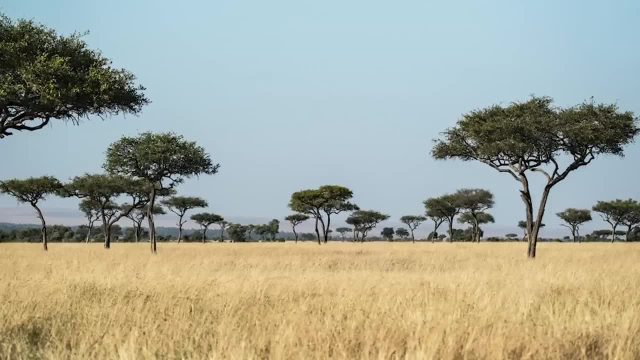 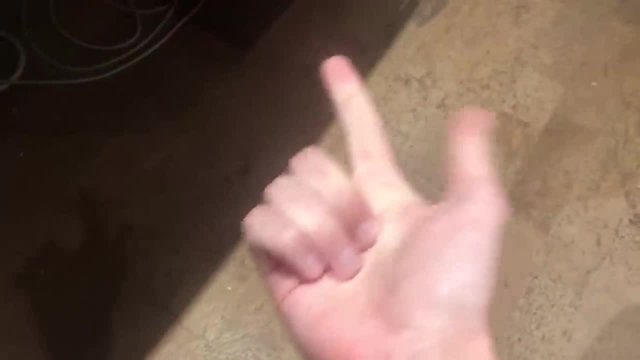 It's likely that counting was the first sign language ever invented, which is a big loss to all the deaf cavemen out there. They could only count at each other. That's good up to 10,. ok, I lied, it's actually good up to 1024 numbers. but come on, you know it's 10.. And humans are big boys now and need 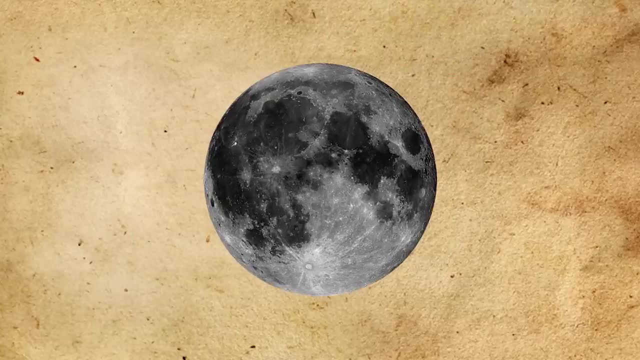 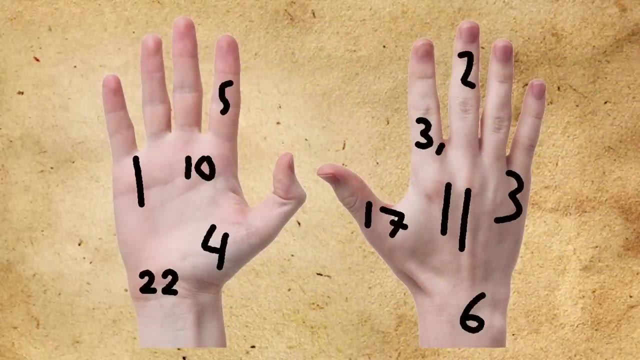 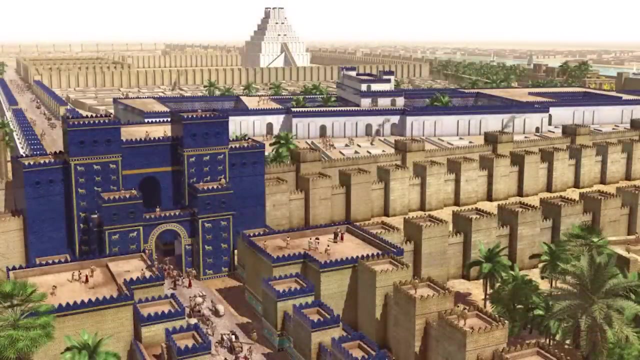 to count, um, I don't know, the moon I guess, Which happens to be in cycles of 30 days. I have an idea: let's put numbers under our hands, or at least under animals' hands. Tally's were counted on bones 40,000 years before writing was ever invented. It's negative. 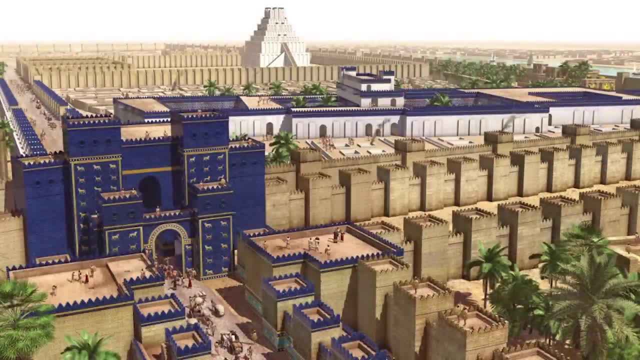 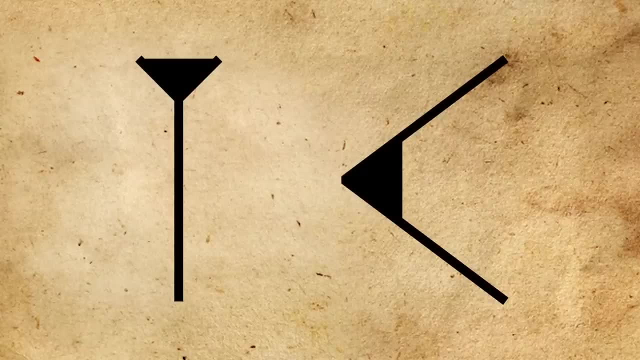 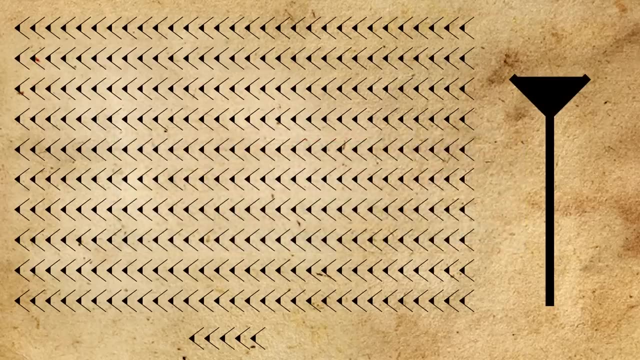 4,000 now. Society was built, clay was harvested and the Babylonians made these things. What a mess. They could only count ones and tens way faster than on hands. but I mean ask them to write down: you know 3051.. Yeah, nice, try guys. At least they kickstarted writing. 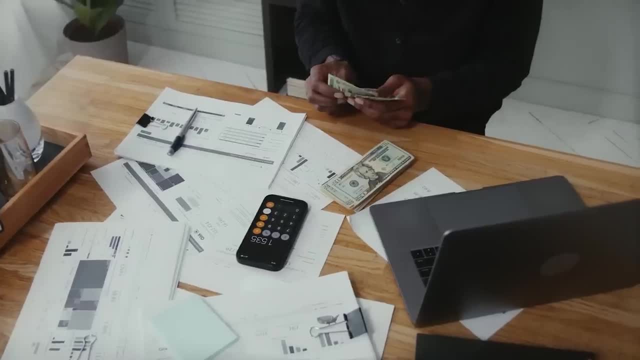 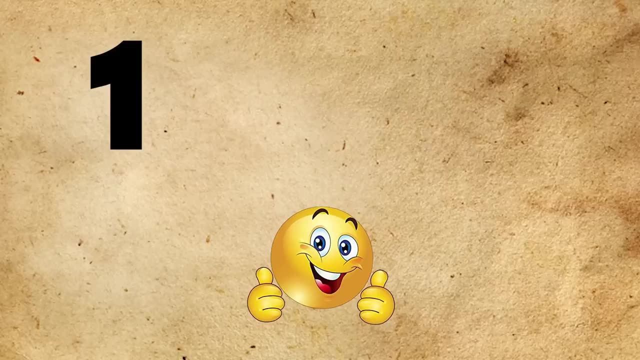 from all their accounting nerd purposes. That's right, all you number crunchers you made writing. Ok, enough fun, get back to my taxes. One is good and two is good, but one and a half. What are you talking about? Around the same time, the ancient Egyptians realized you couldn't. 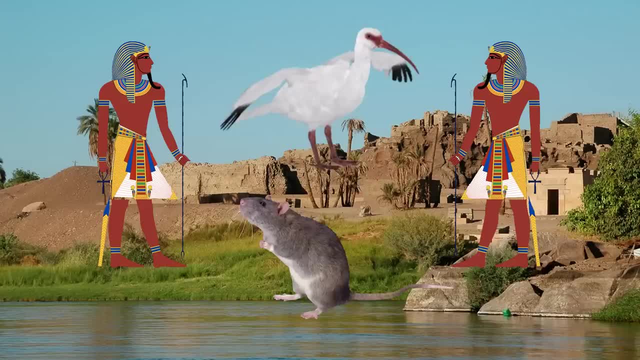 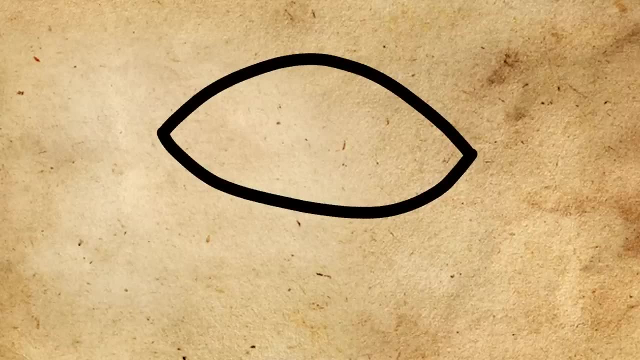 give one pie to two people, or actually a bird or a rat or something. They had an even better way to write numbers, but still awful. What am I looking at? They used this symbol for putting a number on the bottom and only used whole reciprocals, except for two thirds. 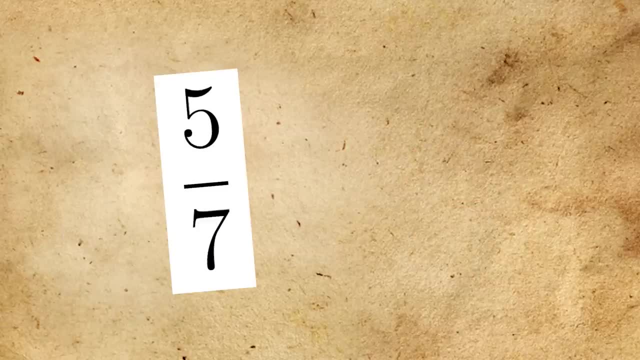 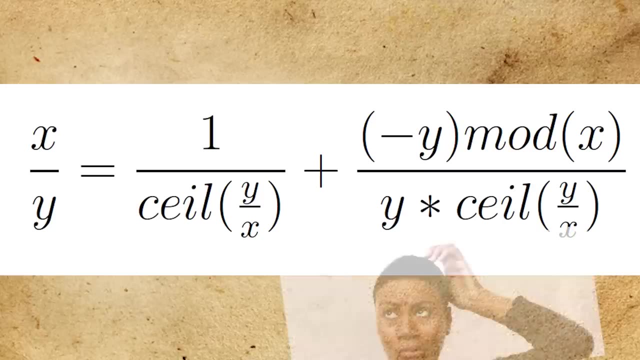 and three quarters, who are apparently special. But what about five, sevenths or eight, ninths? Don't worry, my friend, just add together different reciprocals. According to this, you can always make your fraction. Uh yeah, good going guys, But through a bunch of different systems. 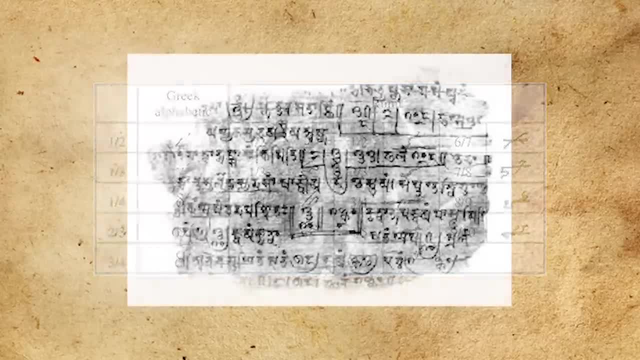 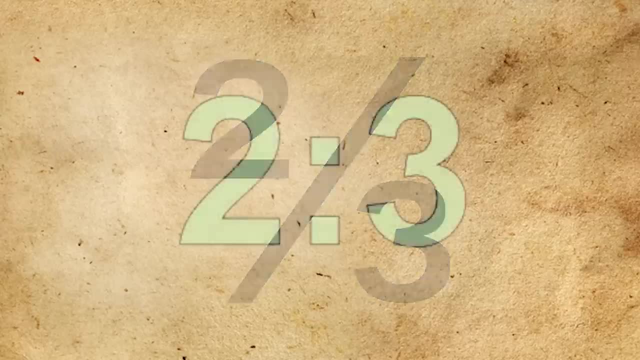 fractions were kind of figured out. Not really, but hey, the Indians got pretty close to the modern day. Those are nice, Almost too nice, as if they're rational, like a ratio between two numbers. What if you don't need this ratio, What? Why would you want that, Maybe? 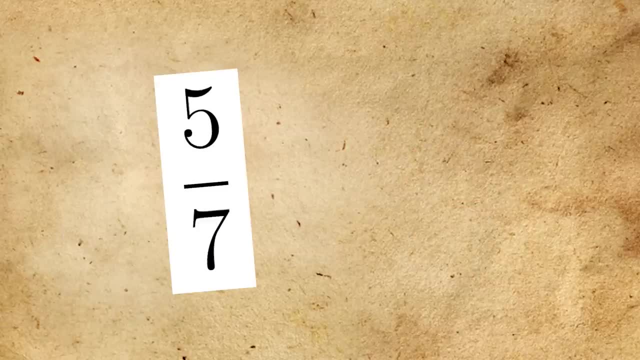 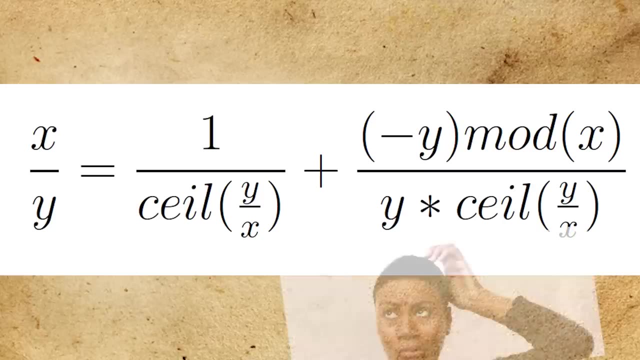 and three quarters, who are apparently special. But what about five, sevenths or eight, ninths? Don't worry, my friend, just add together different reciprocals. According to this, you can always make your fraction. Uh yeah, good going guys, But through a bunch of different systems. 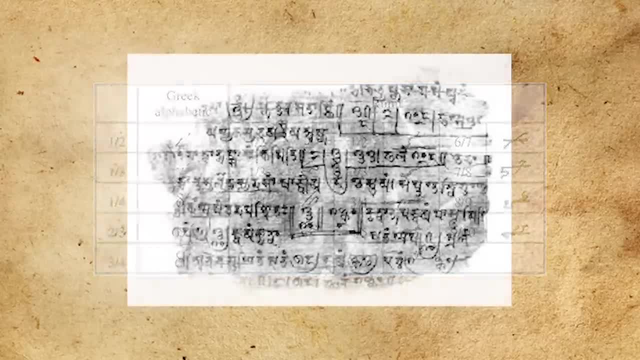 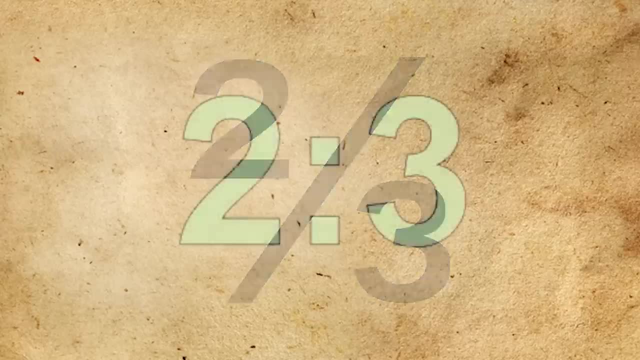 fractions were kind of figured out. Not really, but hey, the Indians got pretty close to the modern day. Those are nice, Almost too nice, as if they're rational, like a ratio between two numbers. What if you don't need this ratio, What? Why would you want that, Maybe? 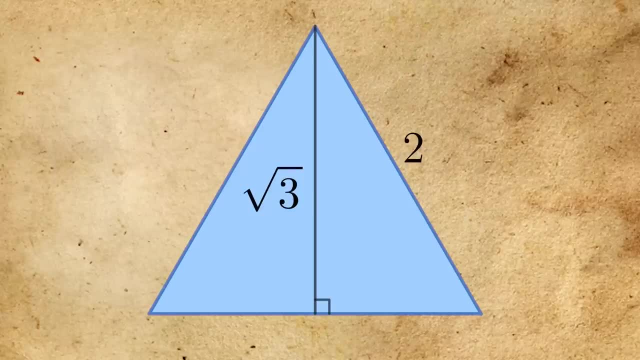 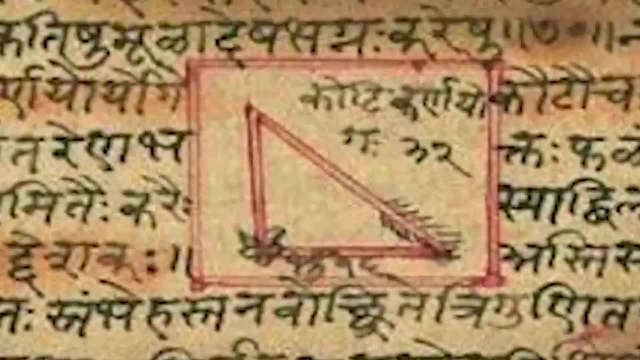 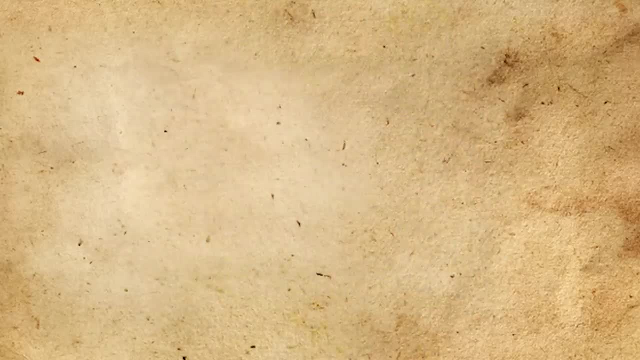 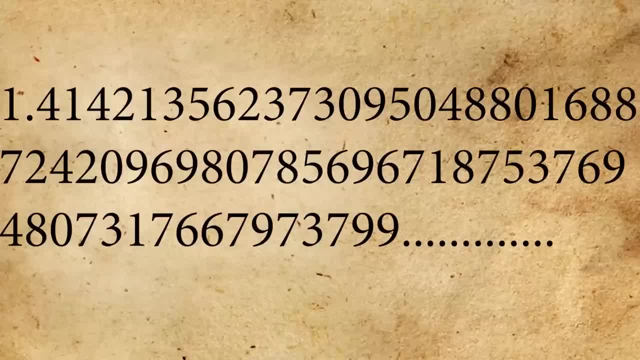 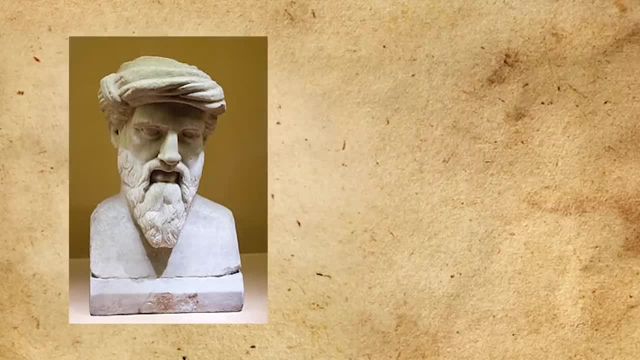 as a perfect, nice way for humans to understand it. That's what happens when you have infinite decimal points. The first guy to realize this fact was someone called Pythagoras. He was the first guy not to try to blindly solve root 2, but instead say: uh, you know what? 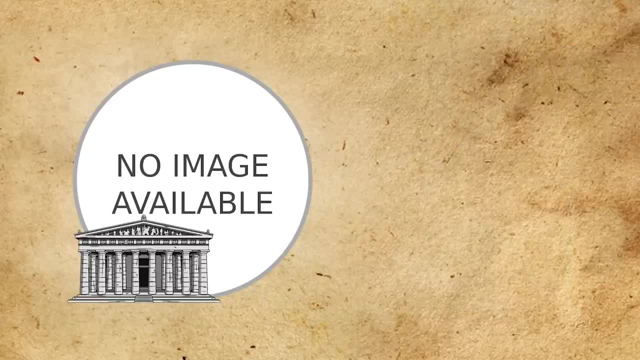 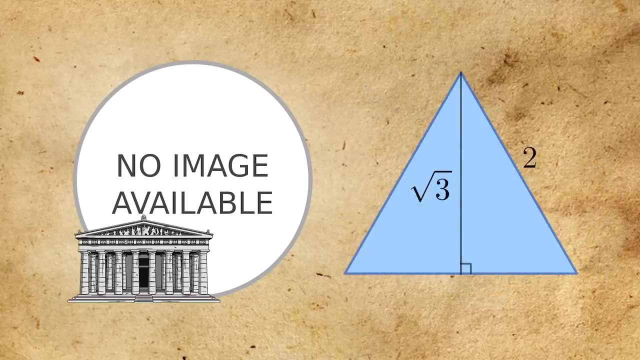 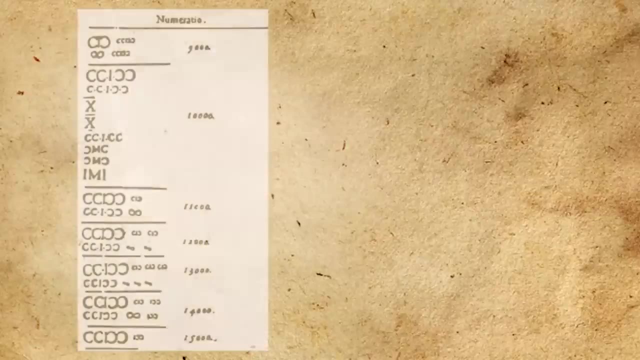 You can't do it except with more logic behind it. Another Greek nerd, Theodorus, made a cool-looking spiral and proved irrationality among 12 more roots, even getting root 3 named after the boy. You know what's even better than Greek maths- Roman maths? You see that they made a a. 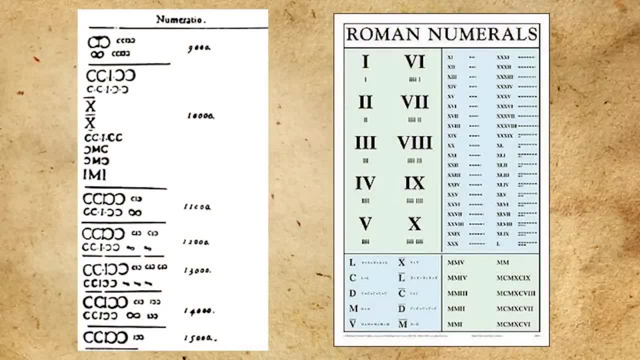 Yeah, never mind. The Romans used strings of letters of value 1,, 5,, 10,, 50,, 100,, 500,, 1,000, up to a million to make up their numbers. But the order highly matters. so IV is 4, but VIII. 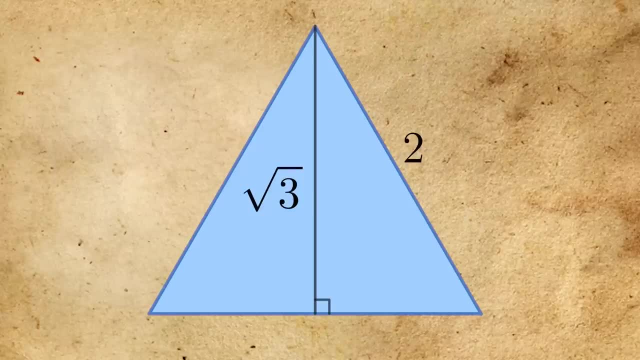 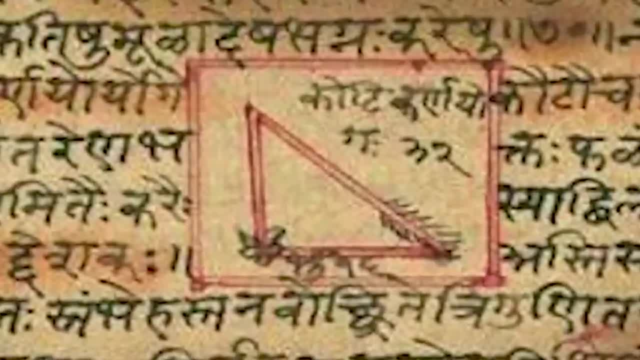 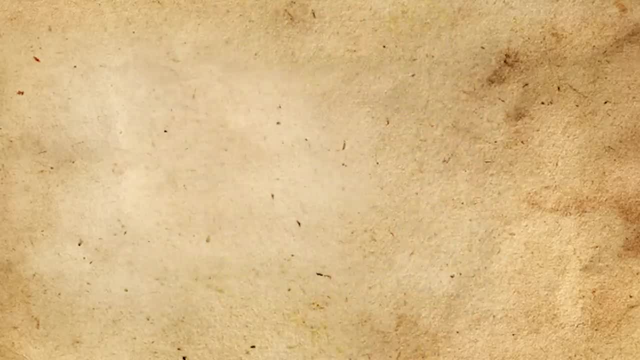 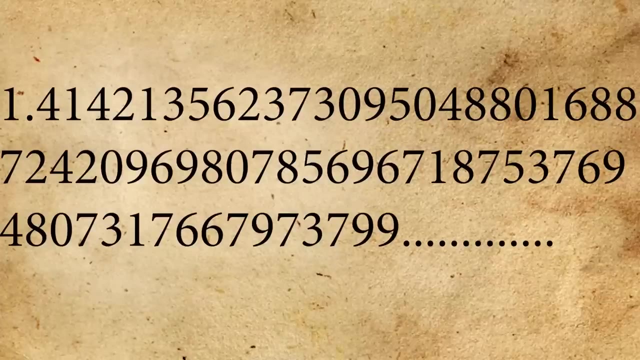 middle of the middle of the middle Santiago of Santa Clara. I'm not talking about them in this book, But it says here that root two is about five hundred and seventy seven over four hundred and eight. WHAT, That's not irrational At. 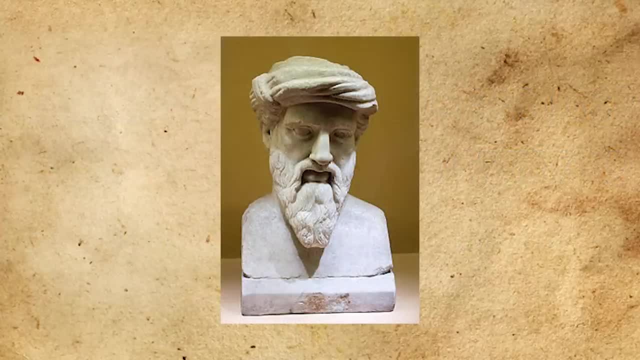 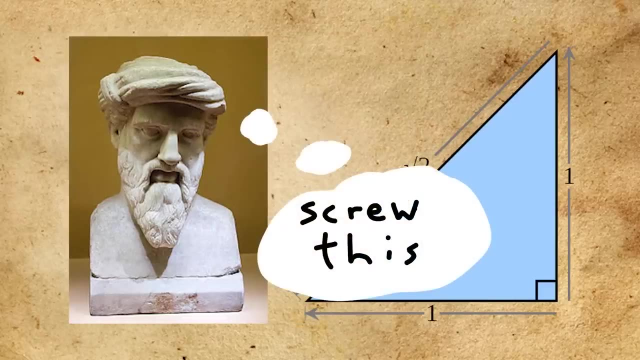 all. Look, you can never express an irrational number as a perfect, nice way for humans to understand it. That's what happens when you have infinite decimal points. The first guy to realize this fact was someone called Pythagoras. He was the first guy to not try. 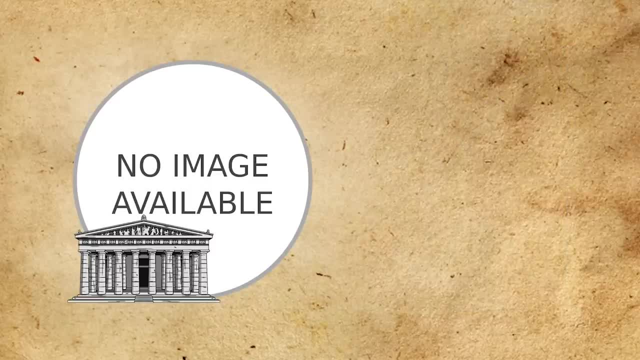 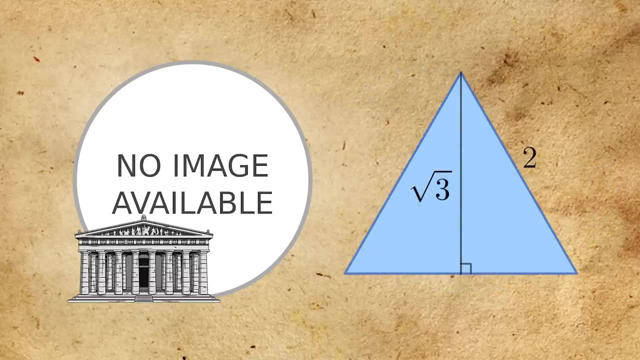 except with more logic behind it. Another Greek nerd, Theodorus, made a cool-looking spiral and proved irrationality among 12 more roots, even getting root 3 named after the boy. You know what's even better than Greek maths, Roman maths? You see that they made a a. 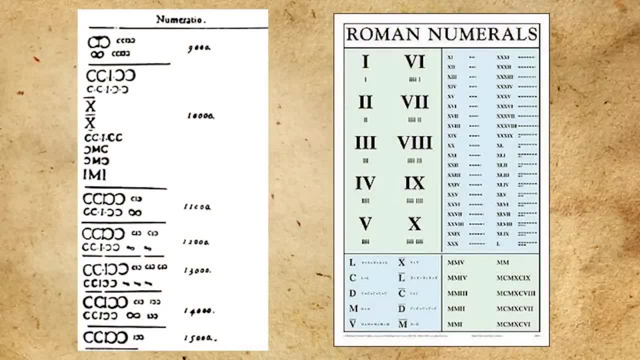 Yeah, never mind. The Romans used strings of letters of value 1,, 5,, 10,, 50,, 100,, 500,, 1,000, up to a million to make up their numbers. But the order highly matters. so IV is 4, but VIII. 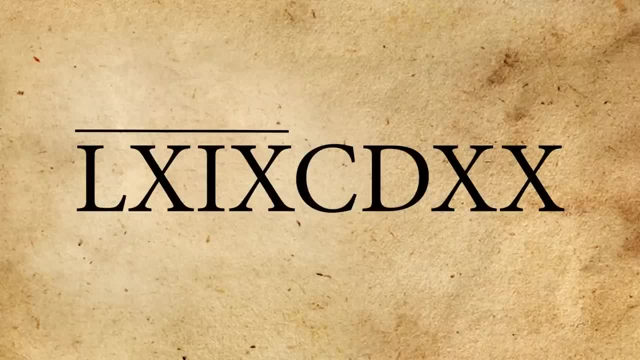 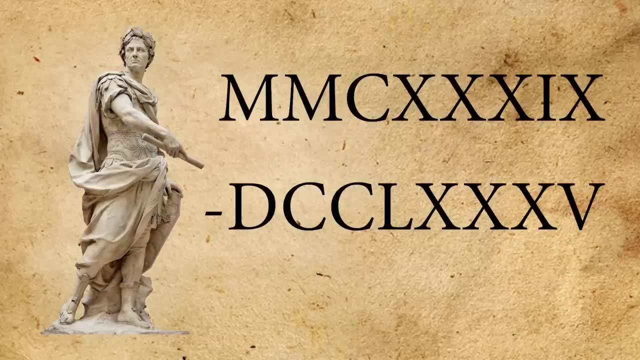 is 8.. What? And this number is, uh, Yeah, I don't know either. Pop quiz for you, Julius. What is this minus this? Yeah, I thought so, And sadly, the Romans made a huge empire, which meant that. 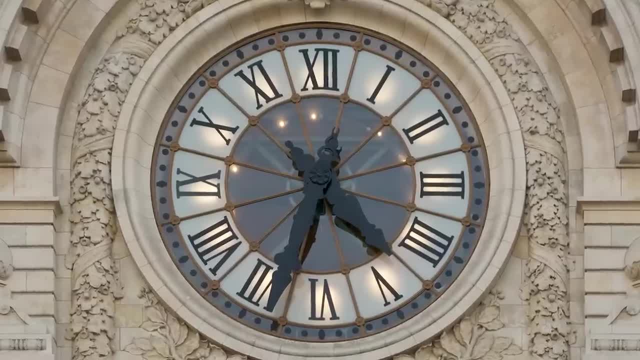 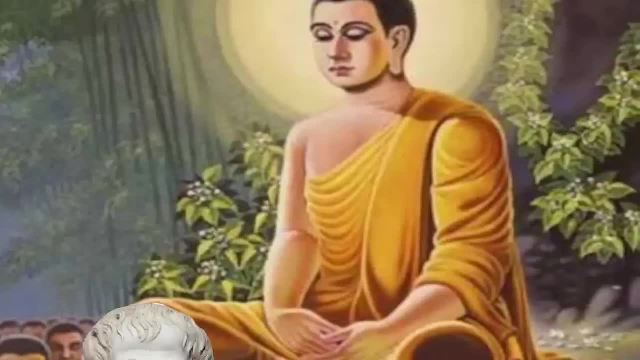 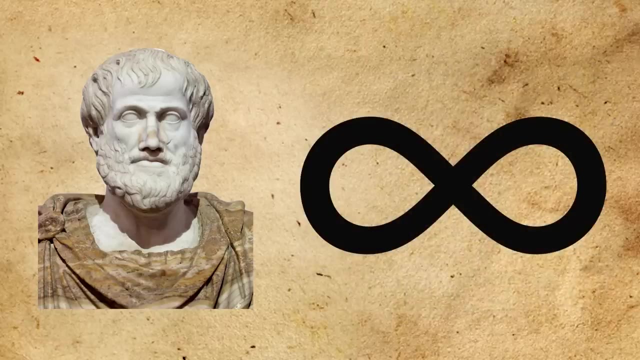 their numeral system lasted in Europe for another thousand years. Truly awful. Ugh, I need to clear my head. Aside from that, let's just sit and think for a while- At least that's what Aristotle did, and he thought about something big, Really big, Infinite. even This wasn't really a mathematical. 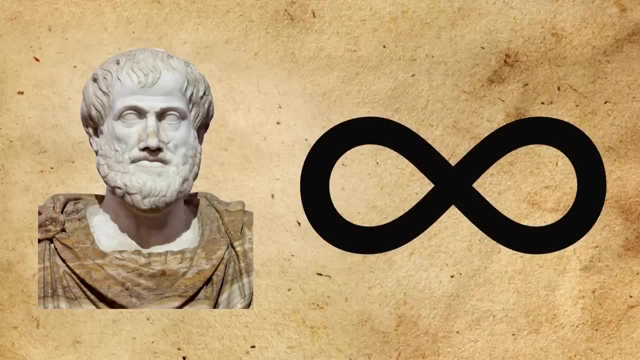 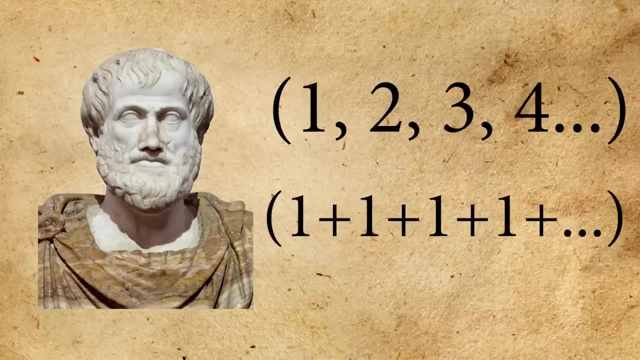 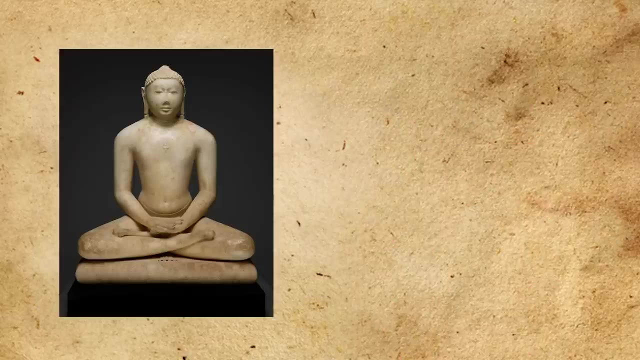 discovery, but more of a philosophical one, And, oh boy, it sure sounds like one. He made up actual infinity entities with completed objects and potential infinity, which is a non-terminating process. Which, Okay, man, that's cool. And around the same time, Jain mathematicians in. 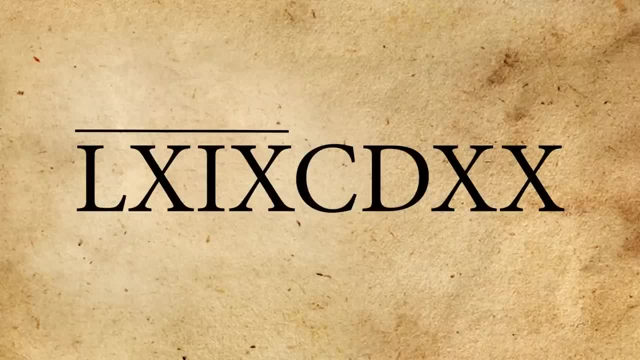 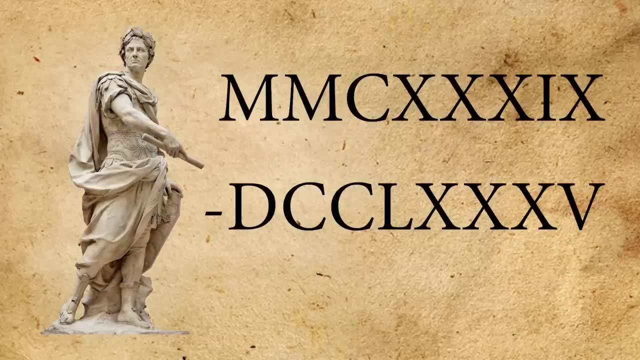 is 8.. What? And this number is, uh, Yeah, I don't know either. Pop quiz for you, Julius. What is this minus this? Yeah, I thought so, And sadly, the Romans made a huge empire, which meant that. 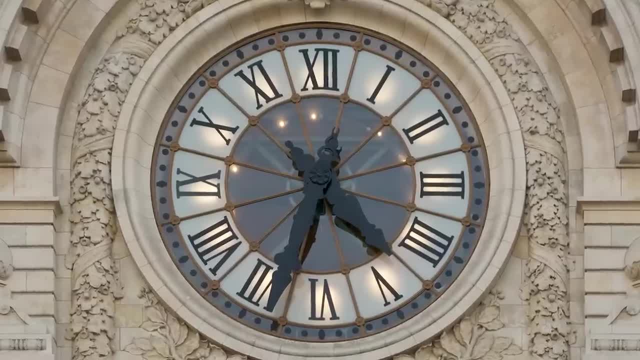 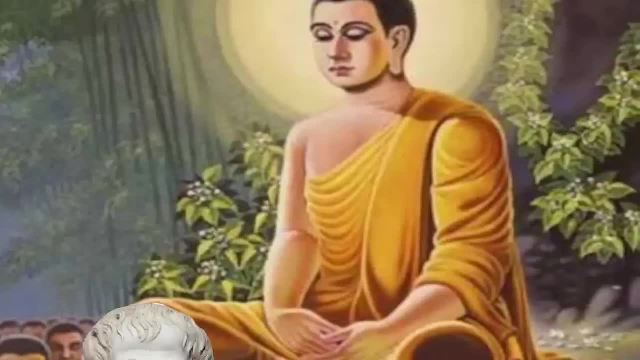 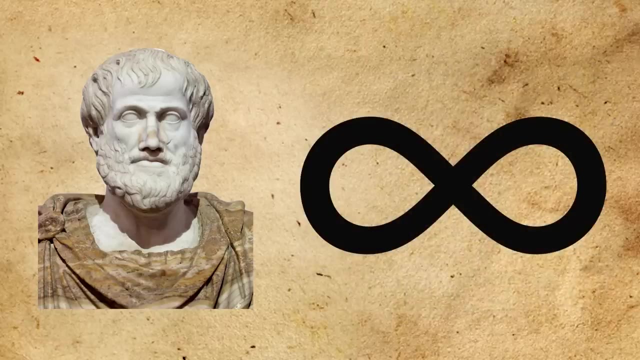 their numeral system lasted in Europe for another thousand years. Truly awful. Ugh, I need to clear my head. Aside from that, let's just sit and think for a while- At least that's what Aristotle did, and he thought about something big, Really big, Infinite. even This wasn't really a mathematical. 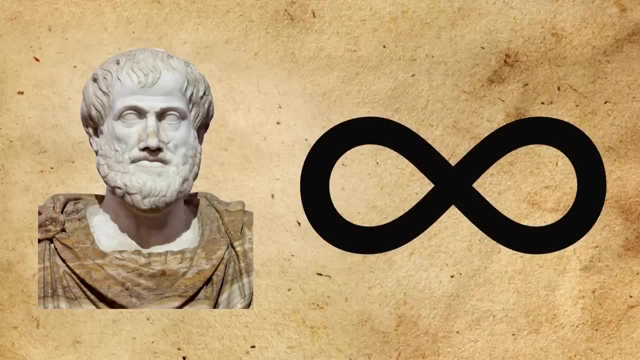 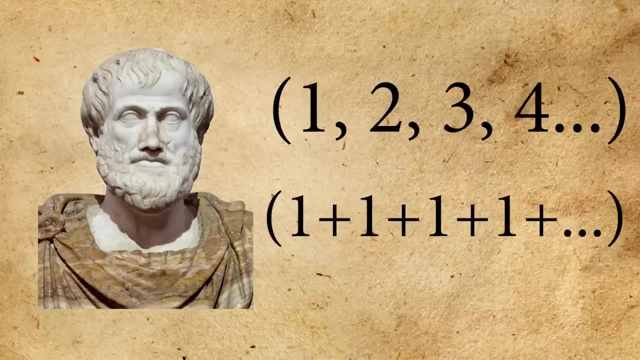 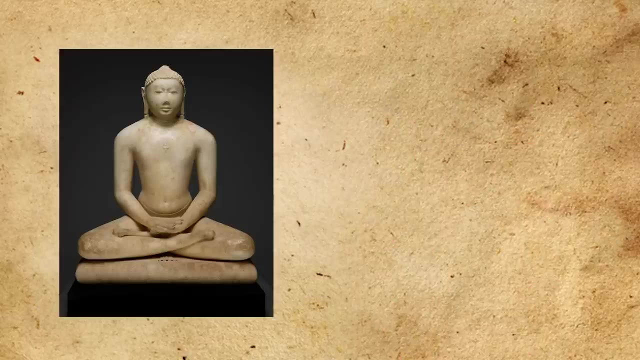 discovery, but more of a philosophical one, And, oh boy, it sure sounds like one. He made up actual infinity entities with completed objects and potential infinity, which is a non-terminating process. Which, Okay, man, that's cool. And around the same time, Jain mathematicians in. 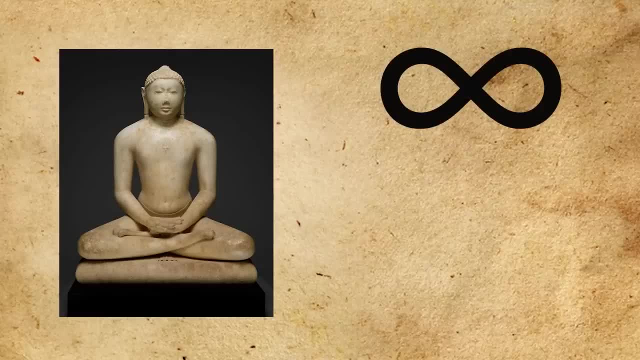 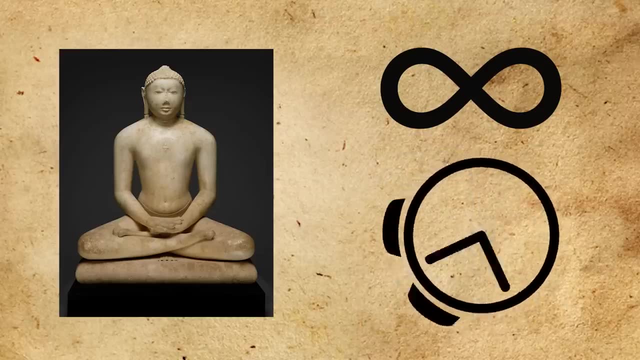 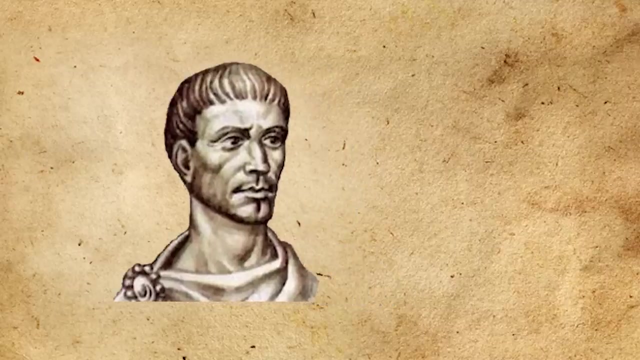 India were loving infinity. They even had 5 types: Infinite in one direction, infinite in two directions, infinite in area, infinite everywhere and infinite perpetually. What the f*** were they smoking? What about something even crazier? Yet another Greek Diophantus thought up an equation. 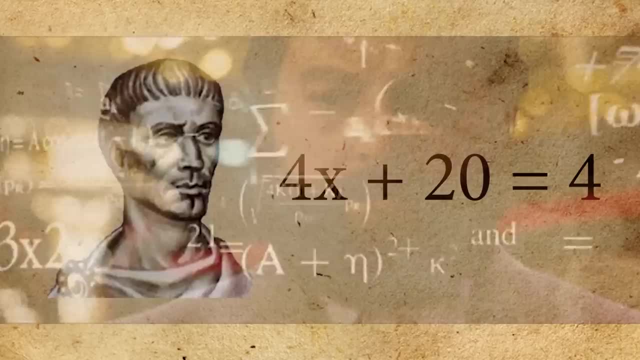 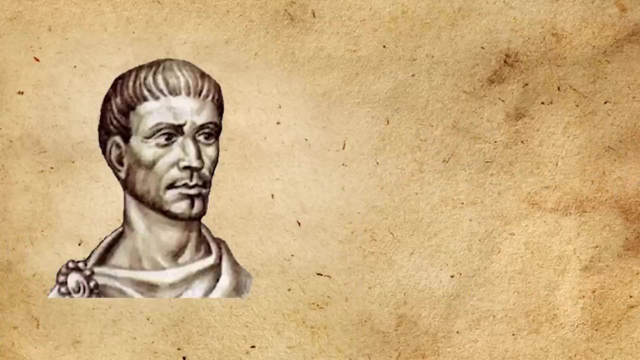 that was basically: 4x plus 20 equals 4.. If you've taken math up to the 7th grade, you'll see that it equals negative 4?. Diophantus thought this was absurd and everyone agreed, Except for the Chinese. in this book They used negative coefficients to find certain areas. 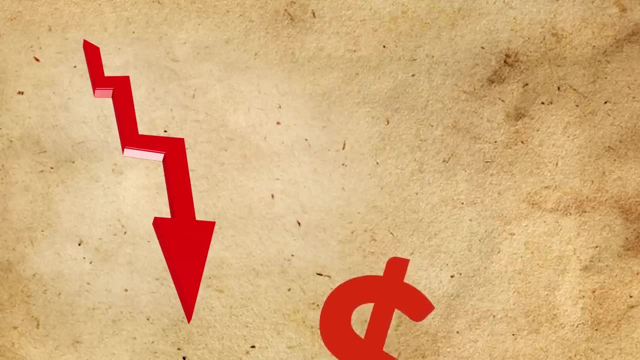 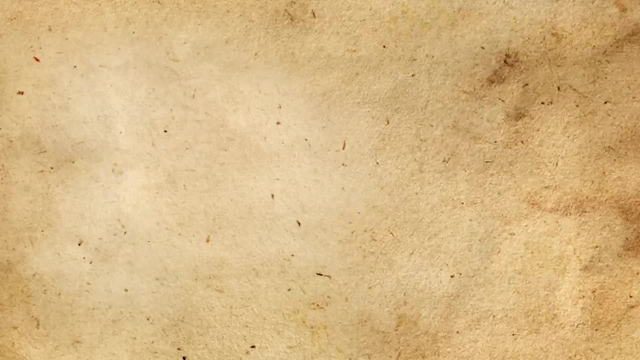 Negative numbers were basically only used to calculate debts. from that point on- Which is actually what I'm in right now- Both European and Indian mathematicians would sometimes just throw away negative results. until the last few centuries, What inspirations We got? pretty much all the. 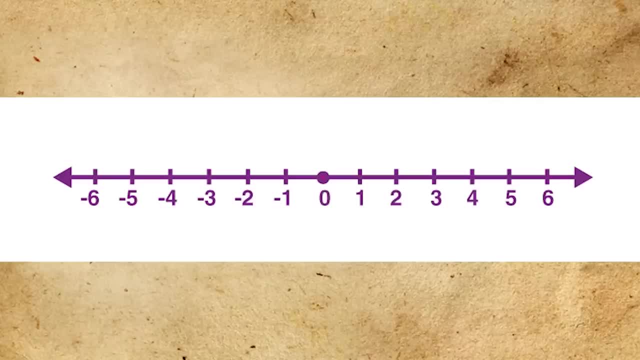 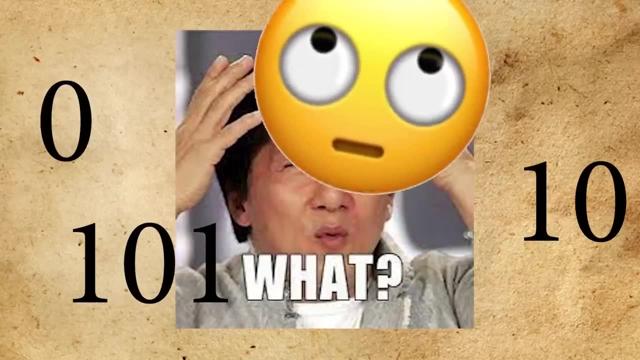 numbers on this number line, but we're missing one. You see that guy in the middle. Their name is zero. And you're probably thinking, blah, blah, blah. how could they know that? Well, they're forgetting zero. It's soooo important, But the Greeks, who love new numbers, said it themselves. 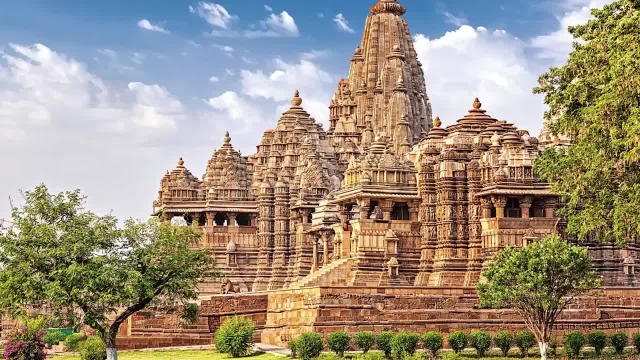 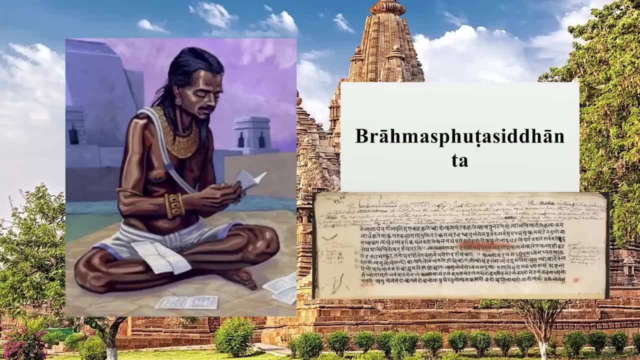 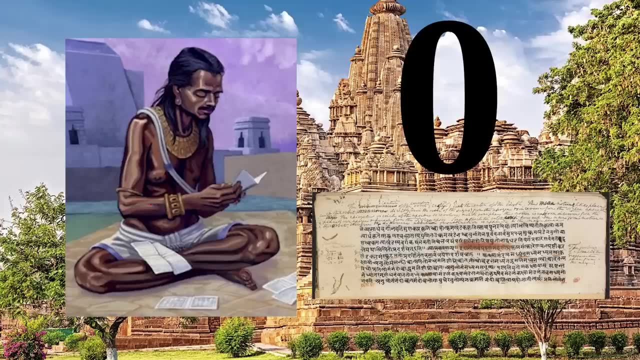 How can nothing be something? Well, they didn't think like that in India, and in 628 AD, Brahmagupta made this new book called. called it's not important. It made our modern understanding of zero and negative numbers, and no one ever used zero anywhere else, except for maybe the. 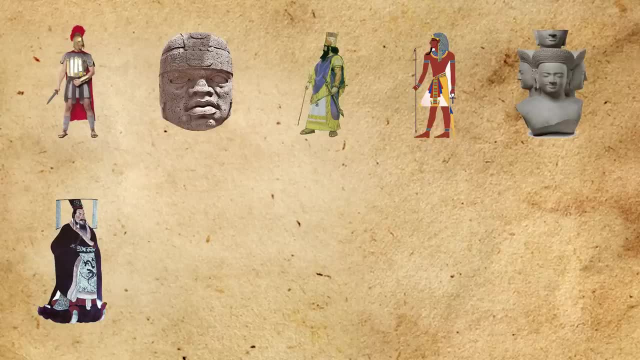 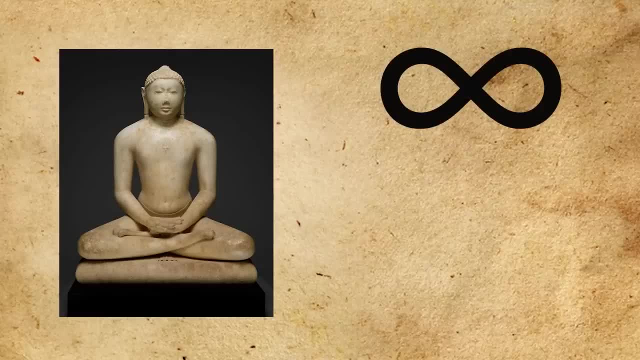 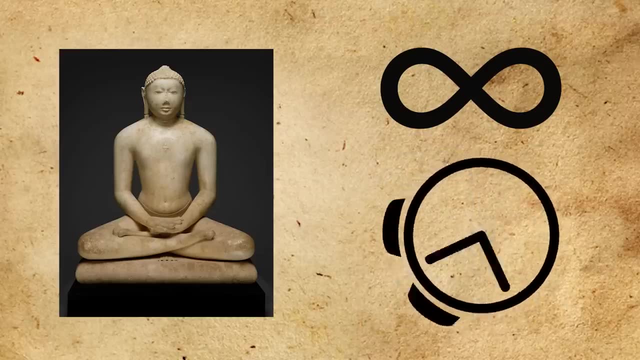 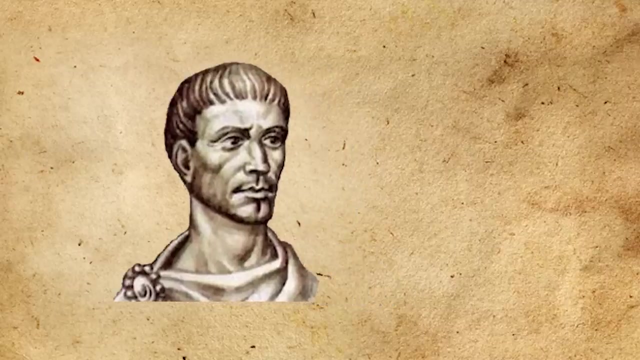 India were loving infinity. They even had 5 types: Infinite in one direction, infinite in two directions, infinite in area, infinite everywhere and infinite perpetually. What the f*** were they smoking? What about something even crazier? Yet another Greek Diophantus thought up an equation. 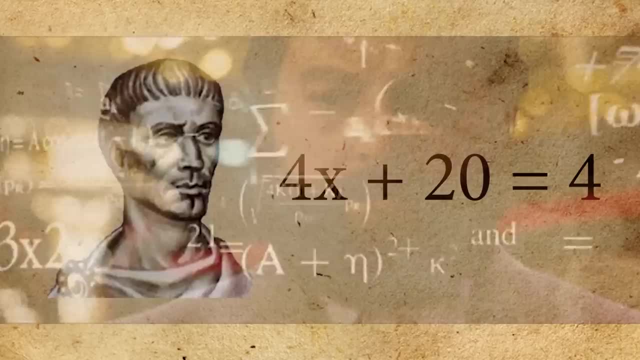 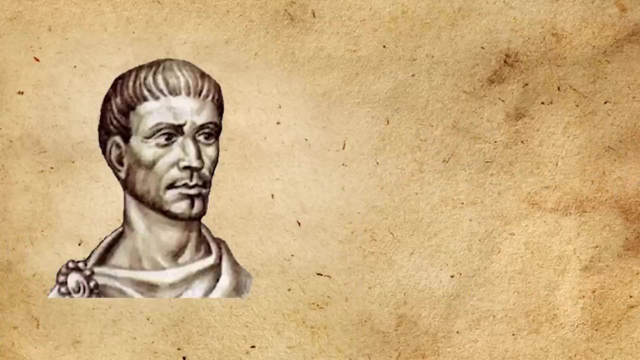 that was basically: 4x plus 20 equals 4.. If you've taken math up to the 7th grade, you'll see that it equals negative 4?. Diophantus thought this was absurd and everyone agreed, Except for the Chinese. in this book They used negative coefficients to find certain areas. 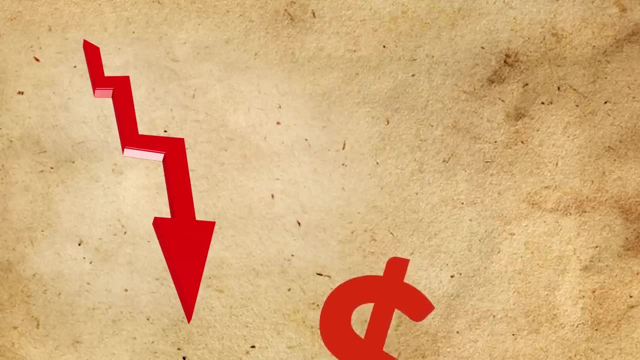 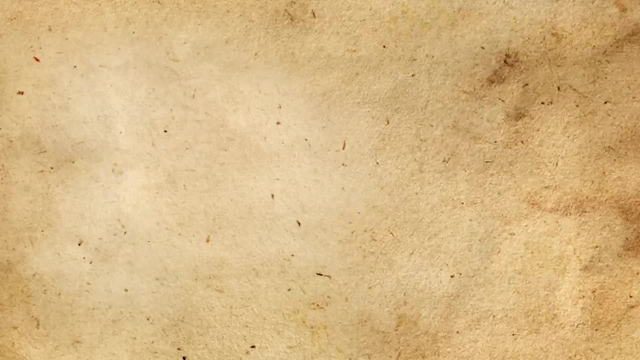 Negative numbers were basically only used to calculate debts. from that point on- Which is actually what I'm in right now- Both European and Indian mathematicians would sometimes just throw away negative results. until the last few centuries, What inspirations We got? pretty much all the. 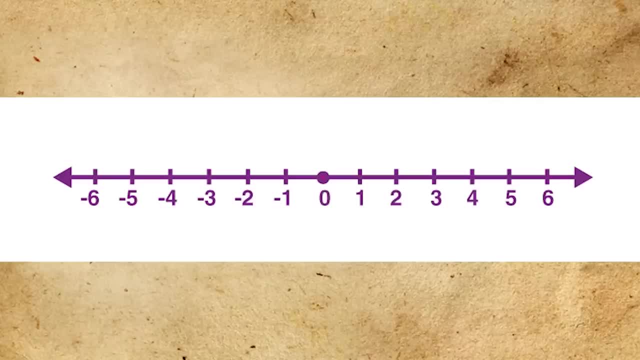 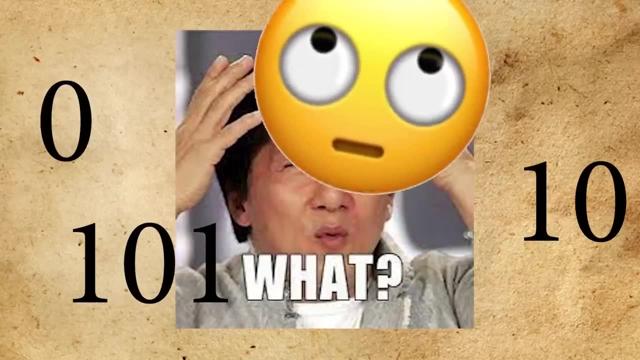 numbers on this number line, but we're missing one. You see that guy in the middle. Their name is zero. And you're probably thinking, blah, blah, blah. how could they know that? Well, they're forgetting zero. It's soooo important, But the Greeks, who love new numbers, said it themselves. 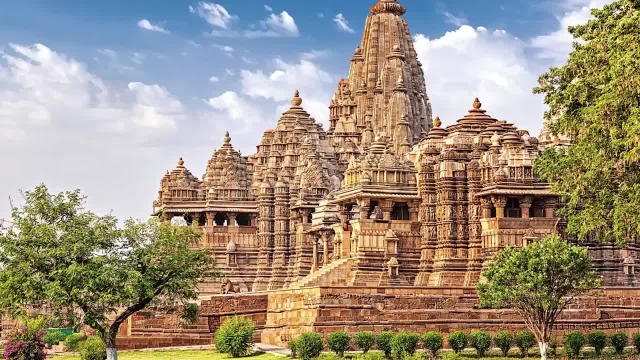 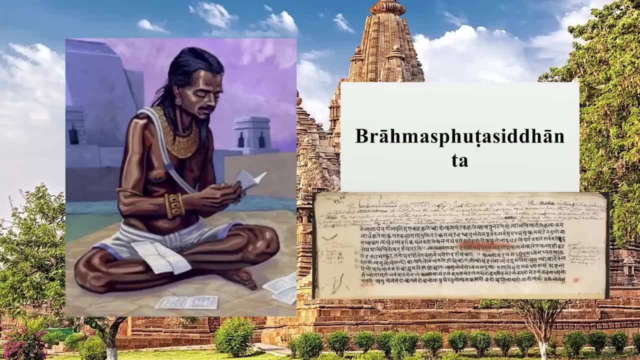 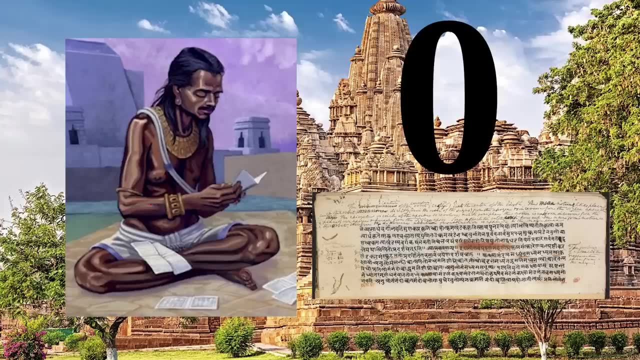 How can nothing be something? Well, they didn't think like that in India, and in 628 AD, Brahmagupta made this new book called. called it's not important. It made our modern understanding of zero and negative numbers, and no one ever used zero anywhere else, except for maybe the. 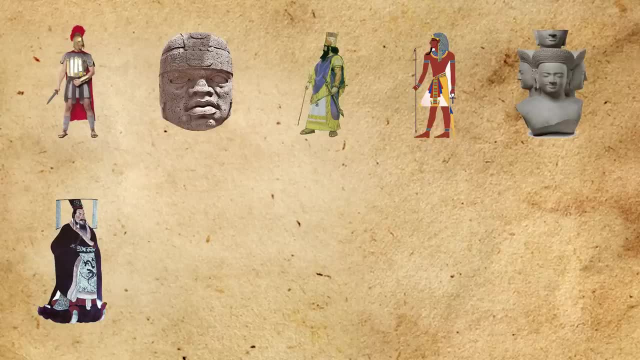 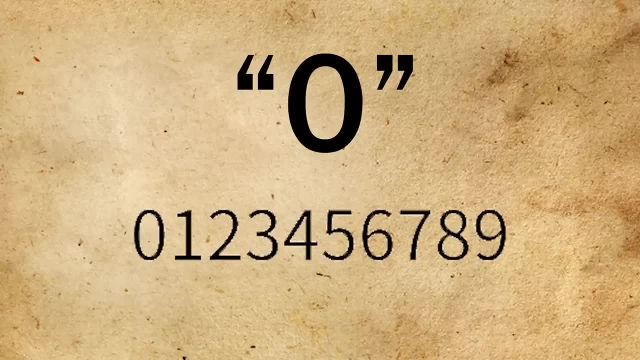 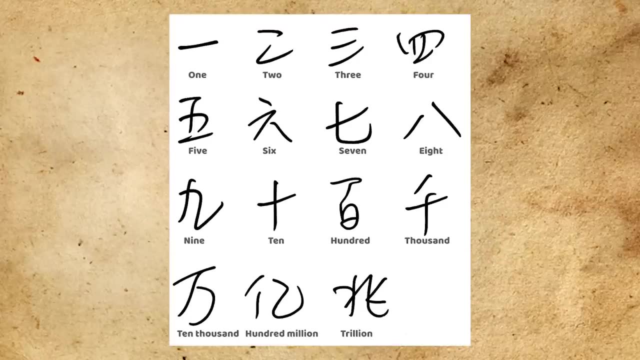 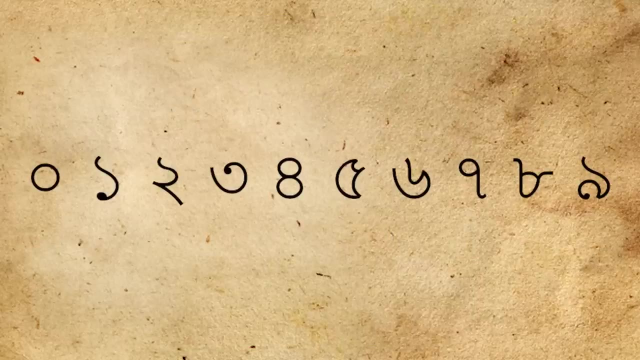 We think of zero like this? it may be because you use the best numeral system out there. No offense, Romans. but let's go through some honorable mentions. Chinese numerals- so fun. they literally just use characters to represent numbers. Just kidding, that's lame, but they did use these cool counting rods. 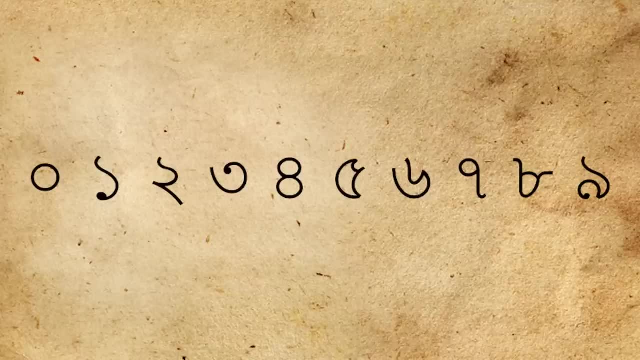 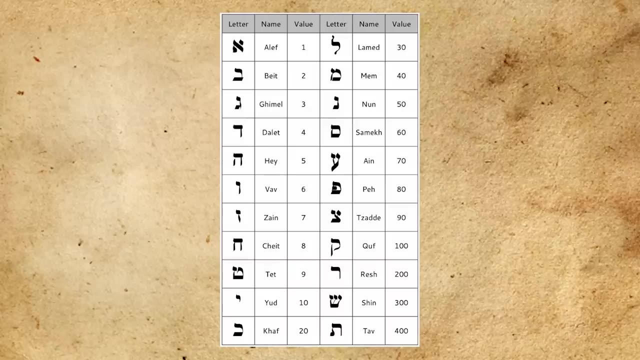 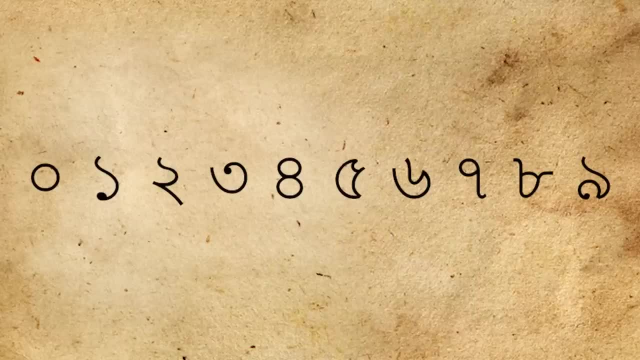 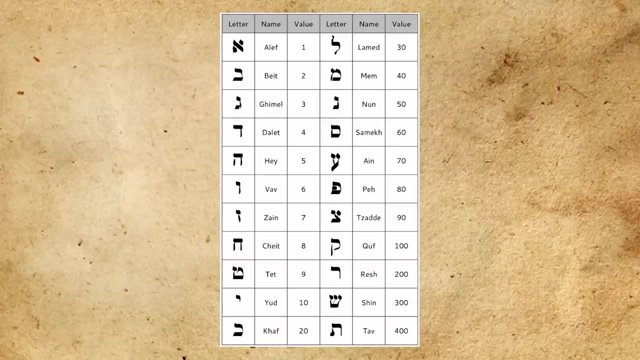 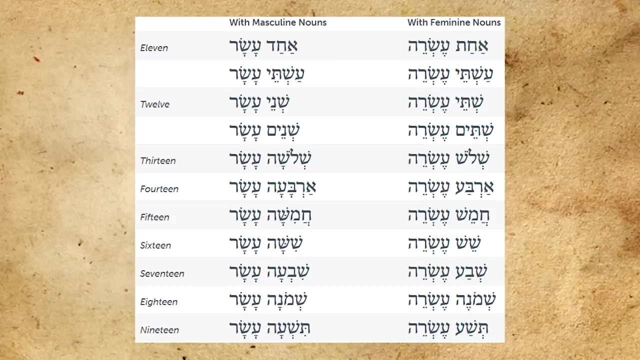 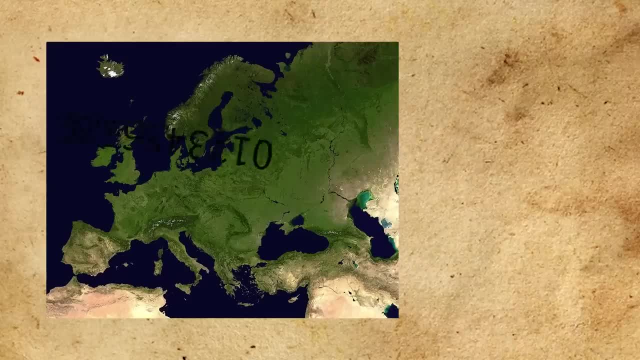 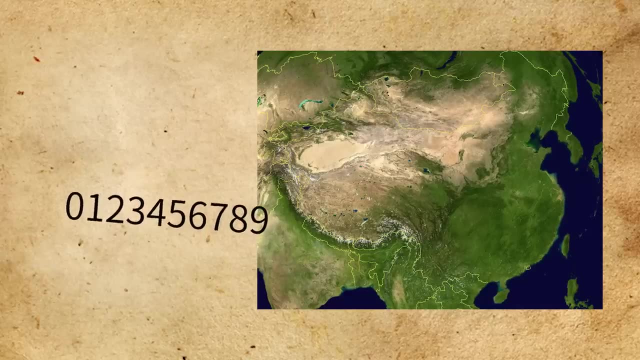 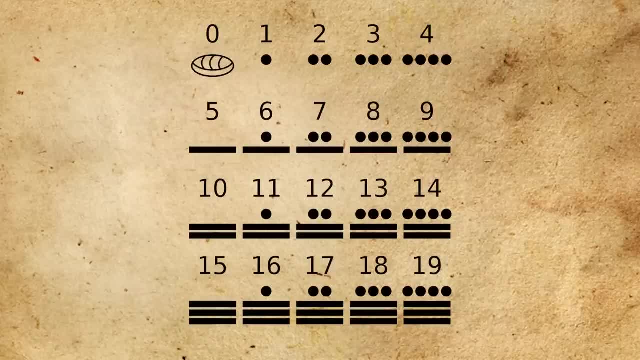 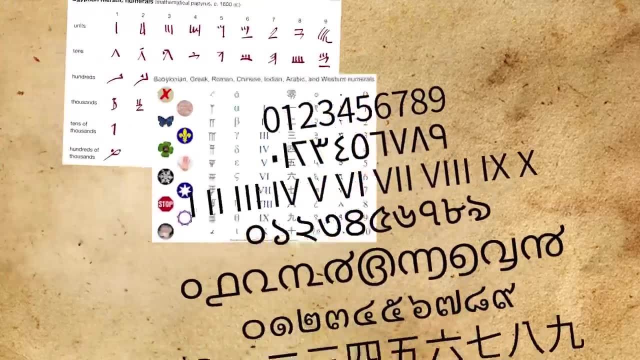 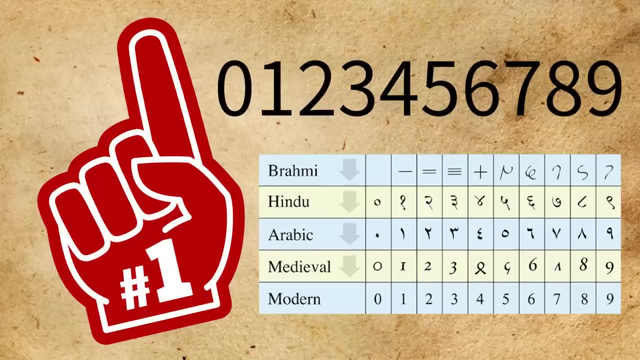 With Hebrew letters and dashes, they make all the numbers they need And Maya numerals. all you need are rods and dots, which makes adding small numbers super easy. I only missed about a hundred other systems, but there can only be one winner. The real GOAT is Hindu, Arabic numerals, or actually any system that has digits 0 and 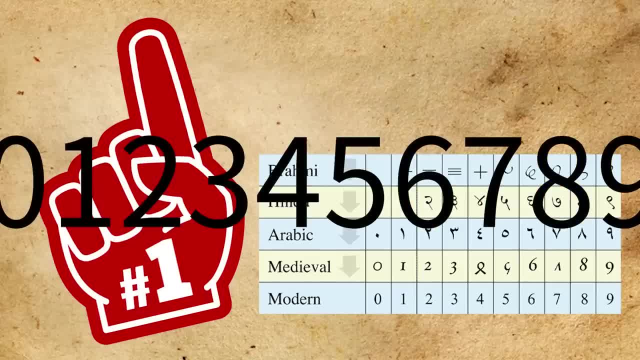 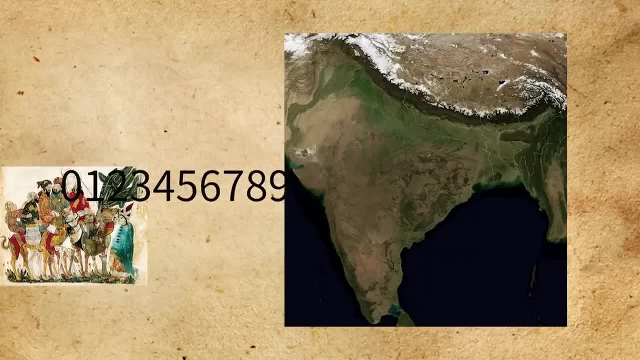 1 to 9, like all of these, Out of all of them, though, these came out on top Starting in India, Arabic traders found them and loved them. The Arabs also love to trade and tell everyone: yeah, We made these. 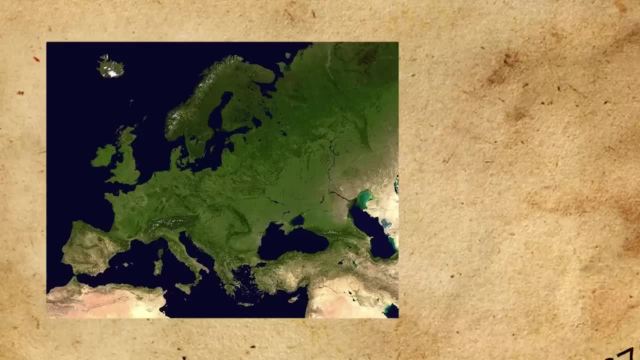 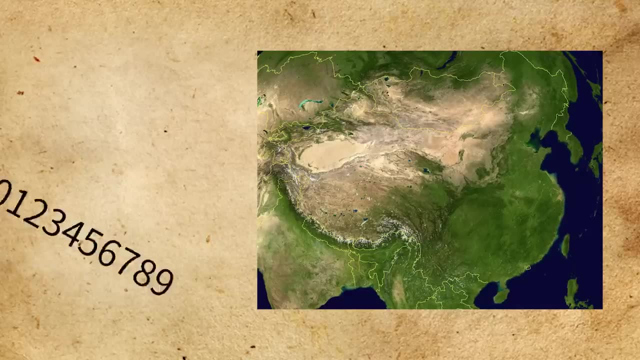 Who cares who made them? because now all of Eurasia is using them. The Europeans were gradually converted, but after the trendsetter Fibonacci started using them, it was all the rage And the Chinese were introduced about a thousand years before they finally gave in and used. 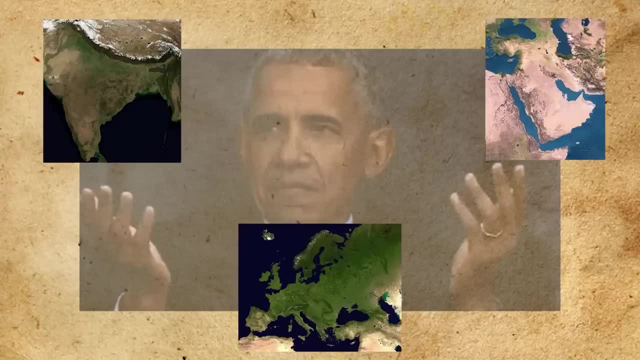 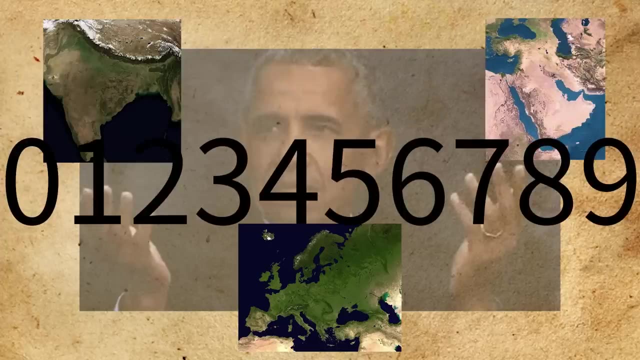 them. Is it a coincidence that India, the Islamic world and the Europeans had a golden age of mathematics after adopting the 0 to 9 system? Absa-lutely Nnnn? Actually I don't know. I don't think so. 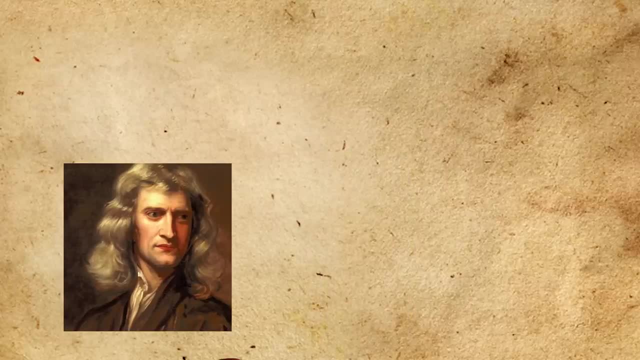 I just think that it's a coincidence, I think that it is, And nothing happens, Until some apple falls on this guy's head. Naturally, he then came up with physics and calculus. Calculus scares a lot of people, but it's really just the math of the infinite. 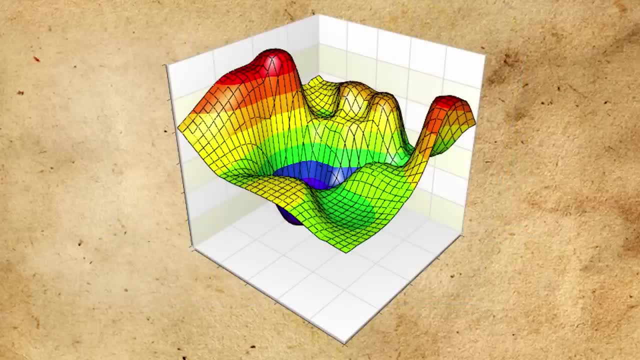 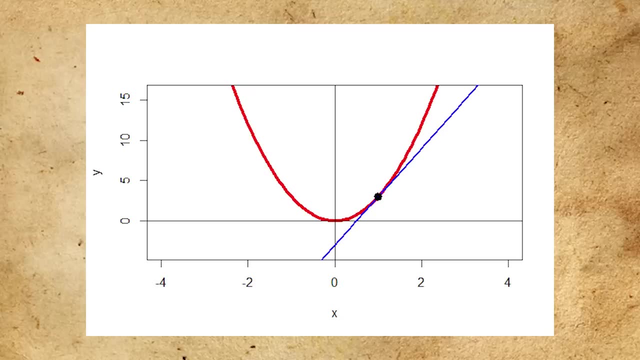 Adding to infinity. adding to infinity, but smooth, or even smoother actually- and instantaneous rate of change. If you're in calculus you hear that and you just put a straight line on a curved one. But if you unblock the non-ascended part of your mind and you hear INSTANT rate of change, 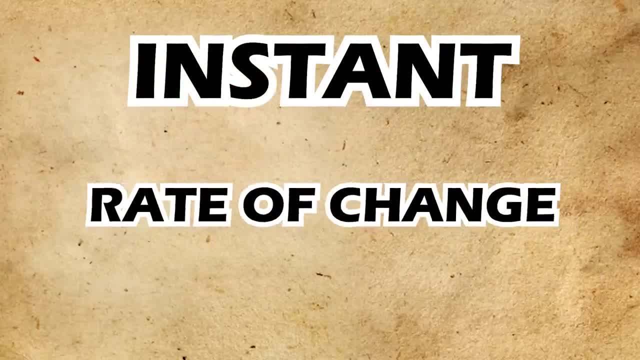 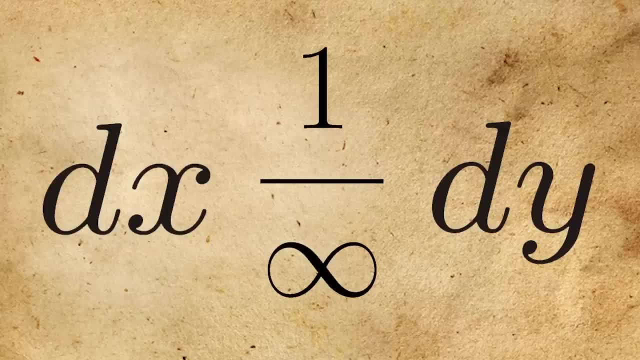 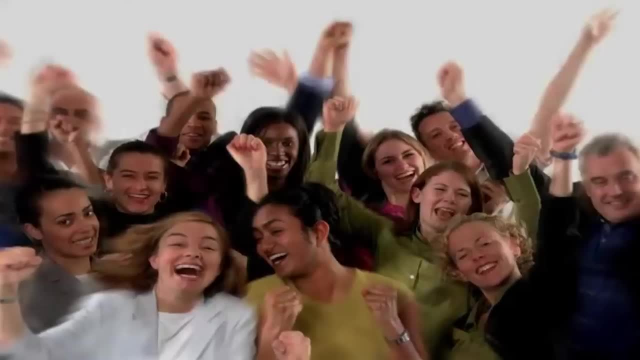 it makes absolutely no sense means there has to be something infinitely small. Newton and Leibniz pioneered the concept of an infinitesimal, usually shown as dx or dy or d-anything really Is something. something when it's basically zero. You tell me Congrats. We finished all the numbers and even threw. 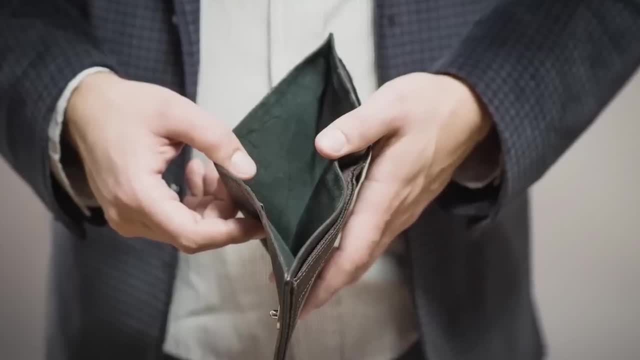 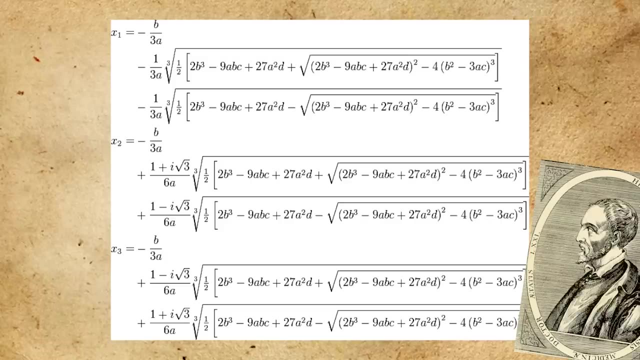 in some concepts along the way. Now there's nothing else for us to do Except make up new numbers. Some Italian boys made up formulas for third and fourth degree polynomials- basically mega-quadratic formulas- and realized that you'll get some crazy numbers out of them. 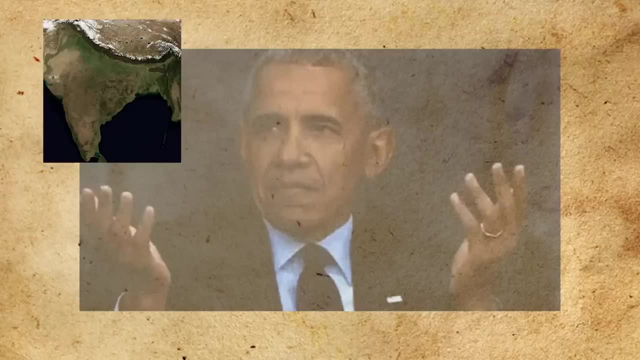 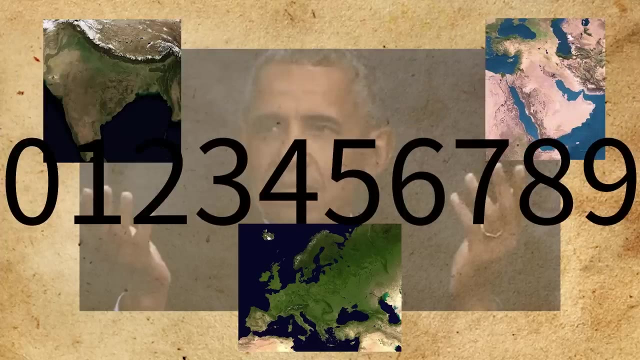 FINALLY GAVE IN AND USED THEM. IS IT A COINCIDENCE THAT INDIA, THE ISLAMIC WORLD AND THE EUROPEANS HAD A GOLDEN AGE OF MATHEMATICS AFTER ADOPTING THE ZERO TO NINE SYSTEM? 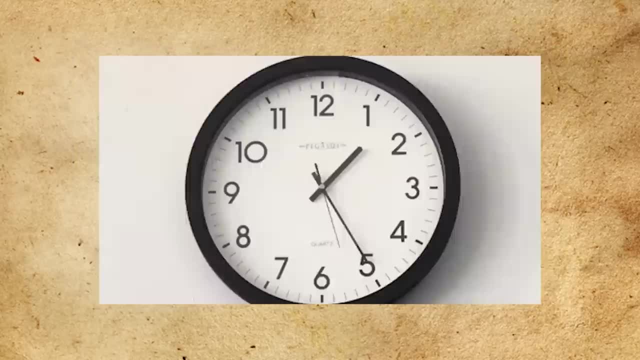 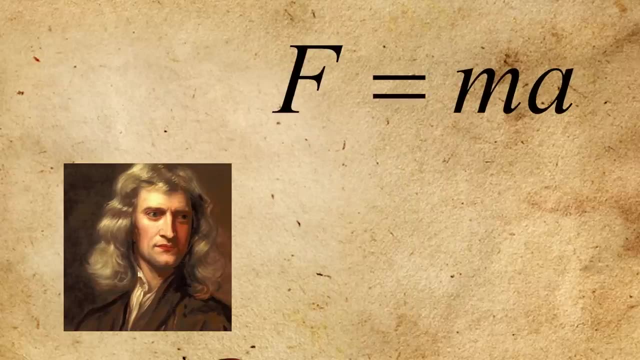 ACTUALLY, I DON'T KNOW. Hundreds of years pass and nothing happens, UNTIL SOME APPLE FALLS ON THIS GUY'S HEAD. Naturally, he then came up with physics and calculus. Calculus scares a lot of people, but it's really just the math of the infinite. 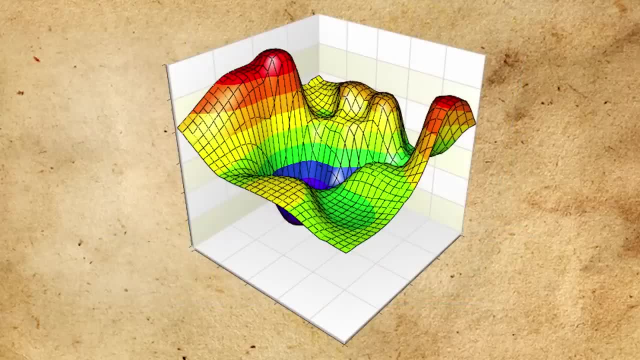 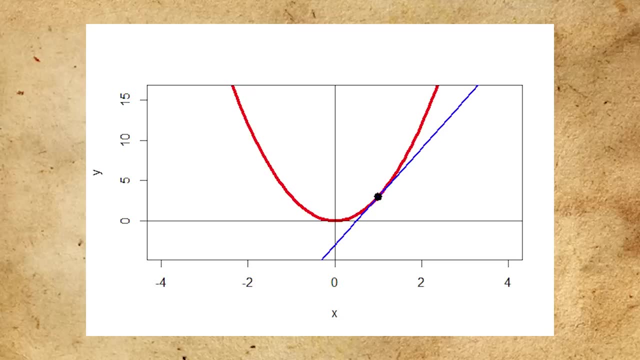 Adding to infinity. adding to infinity, but smooth, or even smoother, actually an instantaneous rate of change. If you're in calculus you hear that and you just put a straight line on a curved one. But if you unblock the non-ascended part of your mind and you hear INSTANT RATE OF CHANGE, 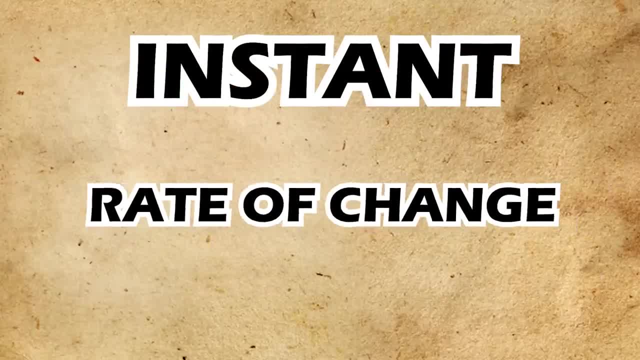 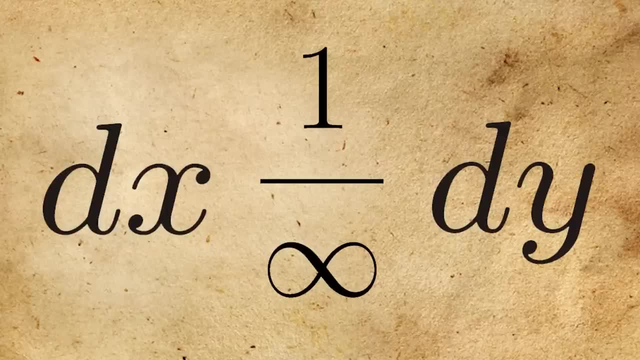 it makes absolutely no sense. That means there has to be something infinitely small. Newton and Leibniz pioneered the concept of an infinitesimal, usually shown as dx or dy or d-anything really Is something, something when it's basically zero. 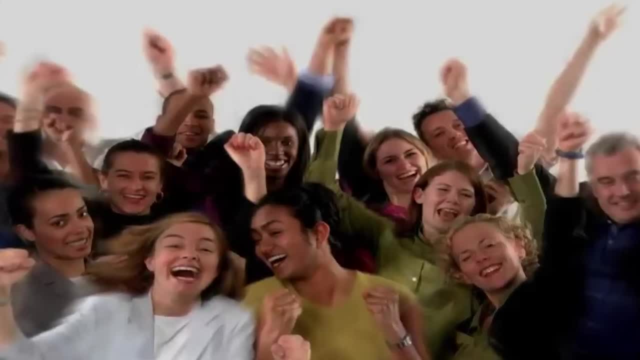 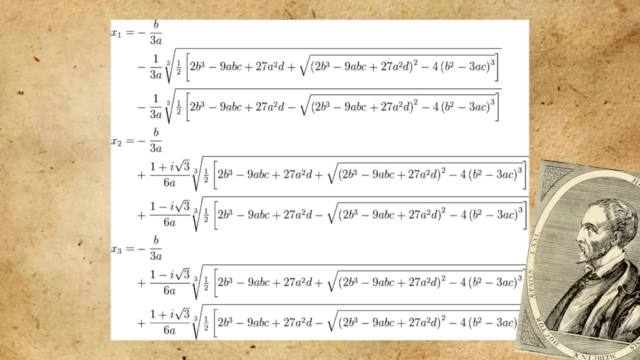 You tell me Congrats. We finished all the numbers and even threw in some concepts along the way. Now there's nothing else for us to do Except make up new numbers. Some Italian boys made up formulas for third and fourth degree polynomials- basically mega. 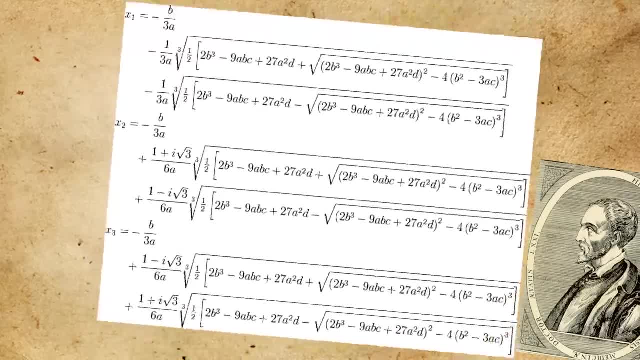 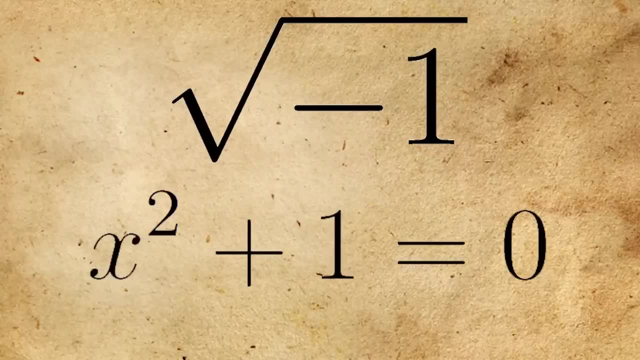 quadratic formulas and realized that you'll get some crazy numbers, Square roots of negative numbers. Do it? Find the square root of negative one? Solve this? You can't, At least not with our numbers. Just make the square root of negative one. let's say I: 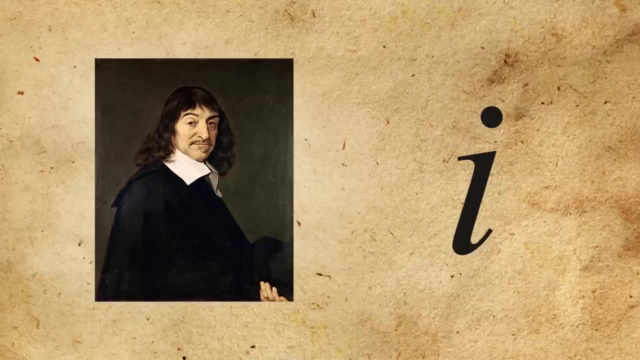 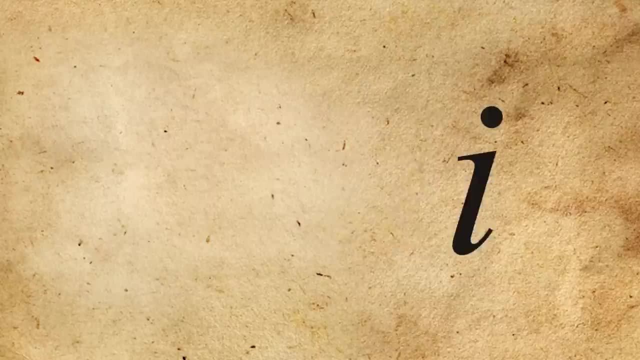 Rene Descartes called these new numbers imaginary. less of a- oh, that's cool like a unicorn imaginary and more of a. you're delusional if you believe in these imaginary, Although the nicer term nowadays are complex numbers. they come in so many flavors adding. 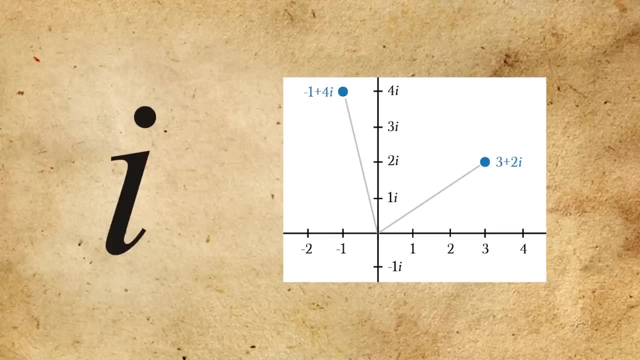 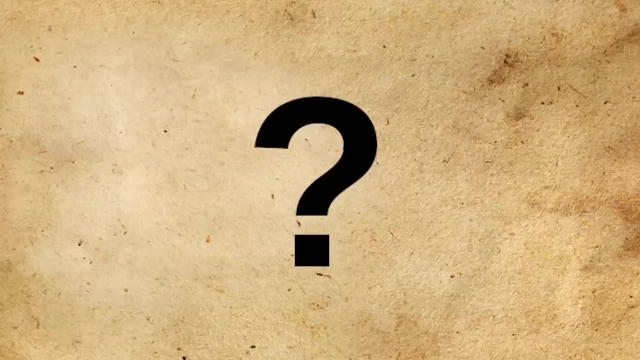 a new access to the number line. Are you team, imaginary or complex? For all the keen viewers out there who've been watching, you may have noticed something missing: A number every person, even kid, knows. That's right, it's pi. 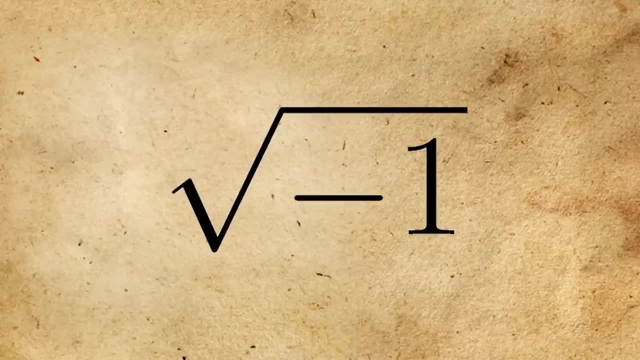 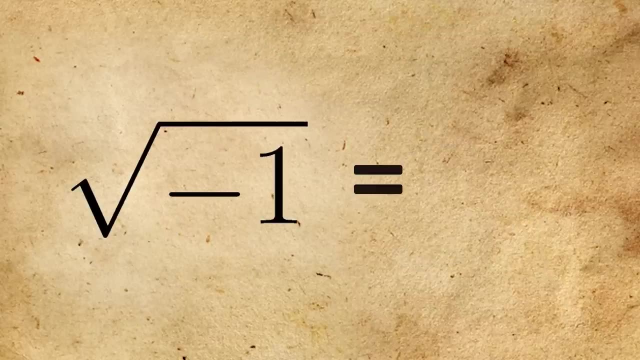 Square roots of negative numbers. Do it? Find the square root of negative one. Solve this. You can't, At least not with our numbers- Just make the square root of negative one. let's say I, Rene Descartes, called these new numbers imaginary Less of a. oh that's. 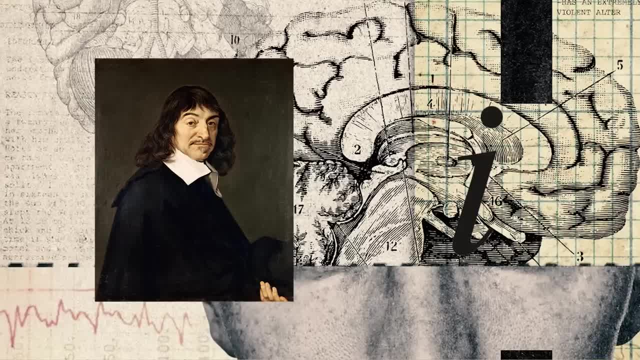 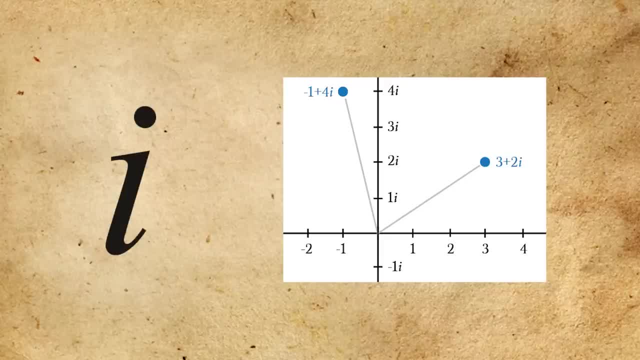 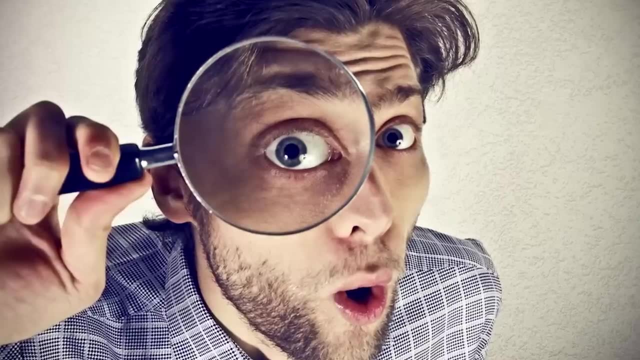 cool like a unicorn imaginary and more of a. you're delusional if you believe in these imaginary, Although the nicer term nowadays are complex numbers. They come in so many flavors, adding a new axis to the number line. Are you team, imaginary or complex? For all the keen viewers out there who've been watching. 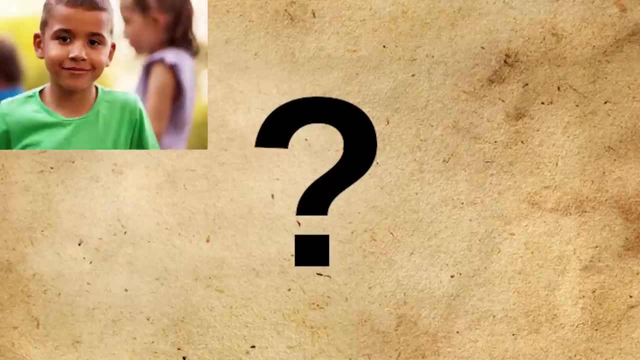 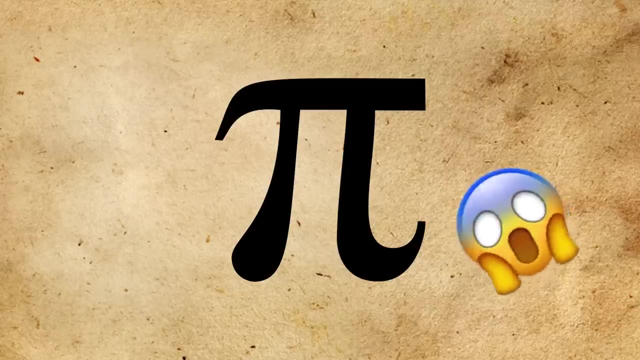 you may have noticed something missing, A number every person, even kid, knows. That's right, it's pi 3.14. blah, blah, blah. OMG, I can't believe you forgot it. After all, isn't that like the ratio of a circle's circumference to its diameter? You're right, but you're. 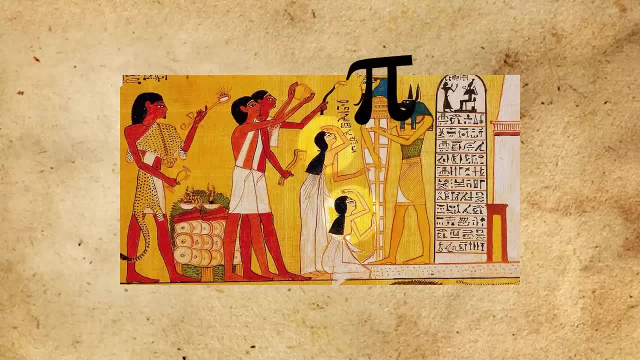 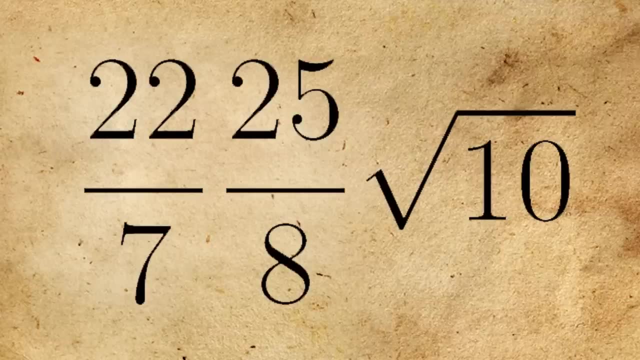 not thinking rational? At least pi isn't. Even though almost every ancient people found something close to pi, like 22 over 7,, 25 over 8, or the square root of 10,, no one proved that it was actually. 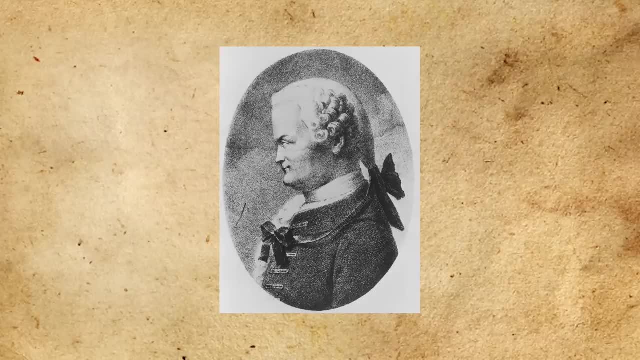 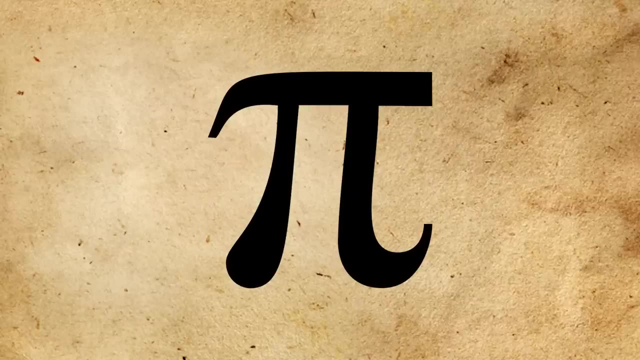 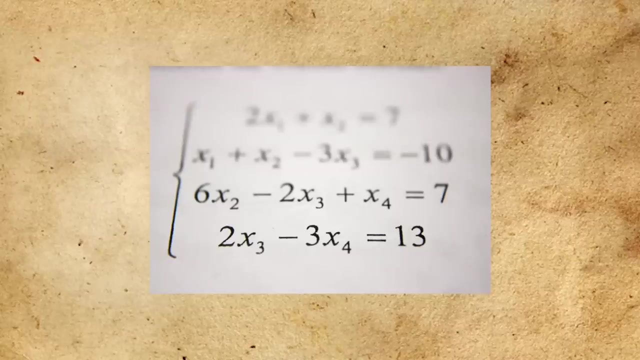 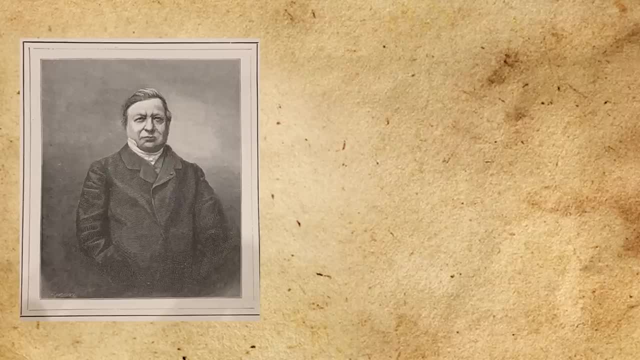 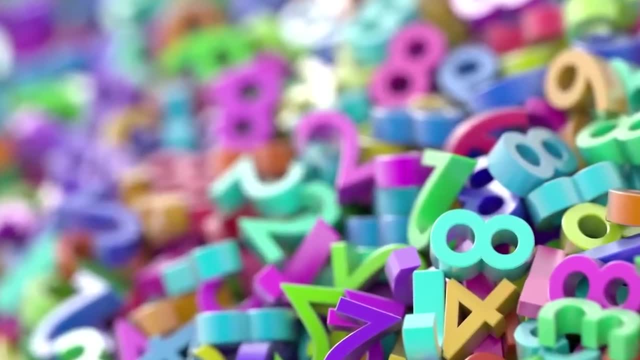 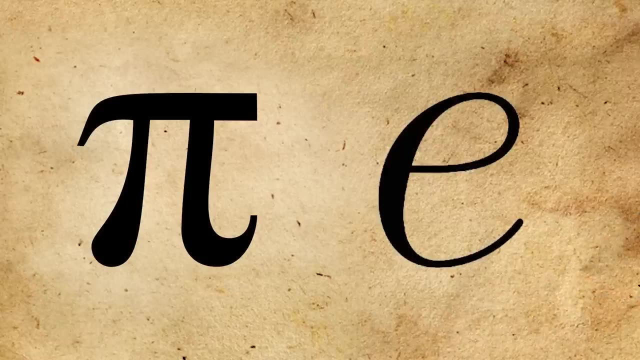 Constant. Most numbers are transcendental, but we only really care about two: Pi and e. But what's e other than the most used letter in English and the least used letter in Mandarin? It's a constant 2.7, blah, blah, blah. named by Leonhard Euler, of course, named. 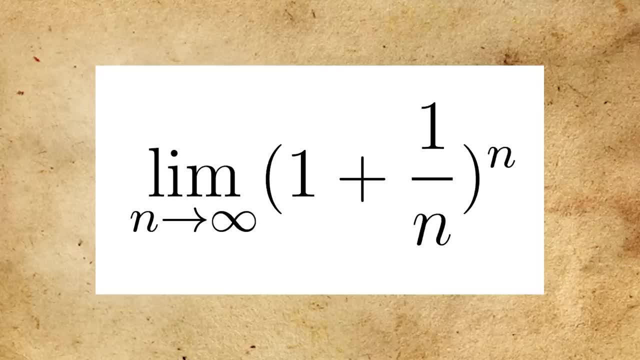 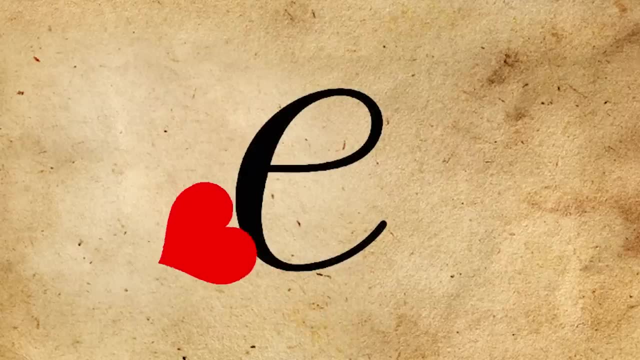 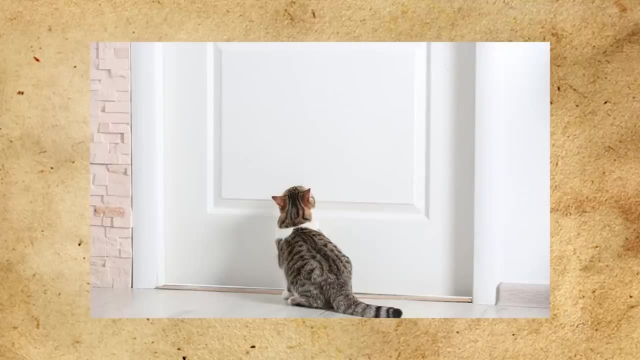 after him, But it is essentially an infinitesimal over 1 multiplied by itself infinitely many times to find like this or this, and mathematicians love it because it's very natural and shows up literally everywhere in math It's like a cat that always shows up when you least. 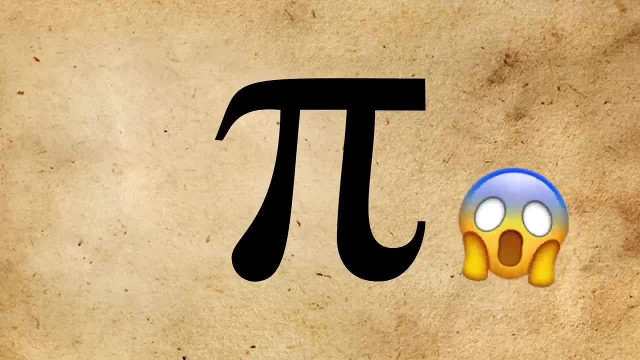 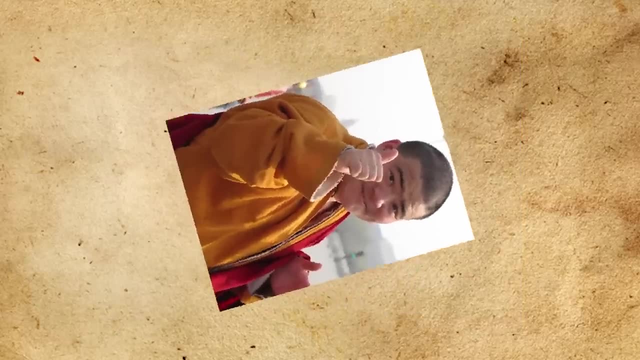 3.14. blah, blah, blah. OMG, I can't believe you forgot it. After all, isn't that like the ratio of a circle's circumference to its diameter? You're right, but you're not thinking rational, Or at least pi isn't. 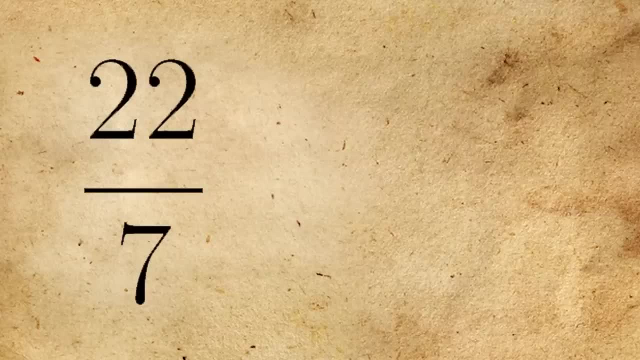 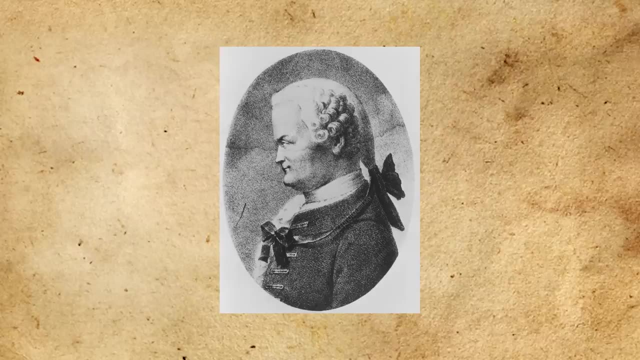 Even though almost every ancient people found it. Even ancient people found something close to pi, like 22 over 7,, 25 over 8, or the square root of 10.. No one proved that it was actually irrational until Johann Lambert did it in 1761, because 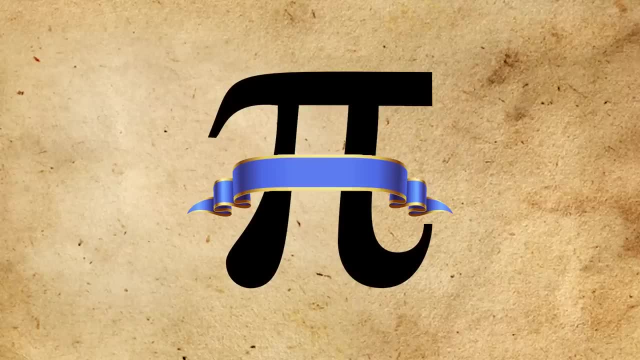 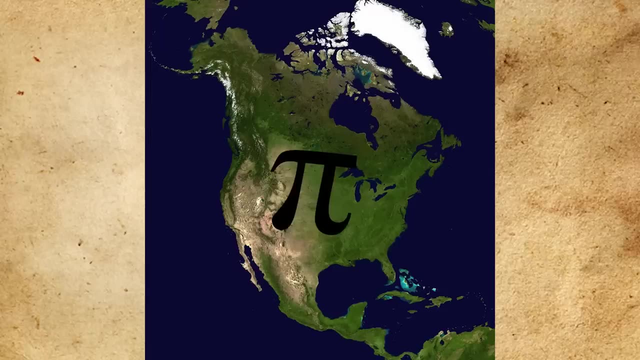 of this. Not only that, pi is even more special than it thinks. with all the attention it gets, Pi is transcendental, which means it spans the whole continent. No, that's not it. It means it can't be written algebraically or as a solution to any polynomial. 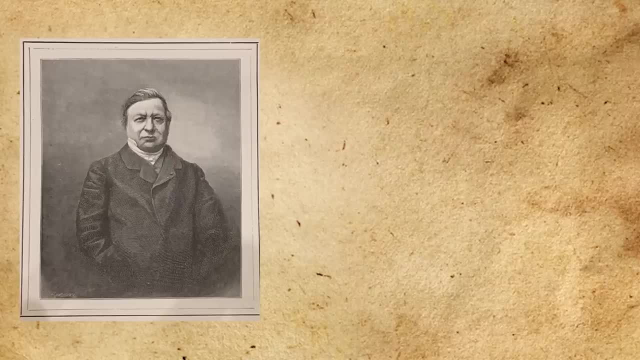 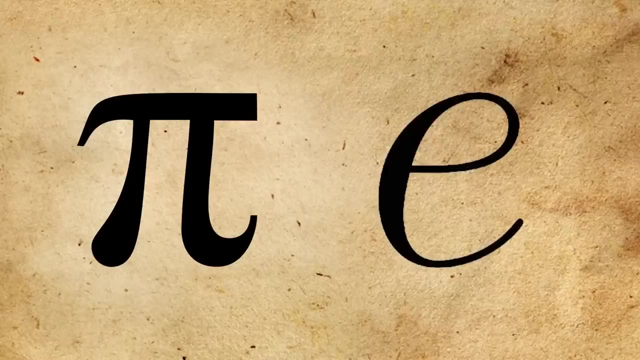 Joseph Louisville wrote this. Louisville essentially birthed this branch of number with the Louisville constant. Most numbers are transcendental, but we only really care about two: pi and e. But what's e other than the most used letter in English and the least used letter in Mandarin? 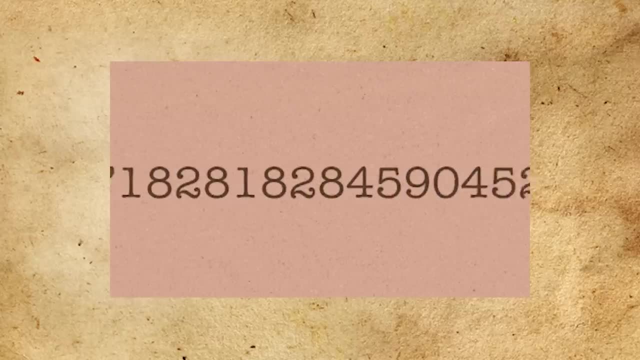 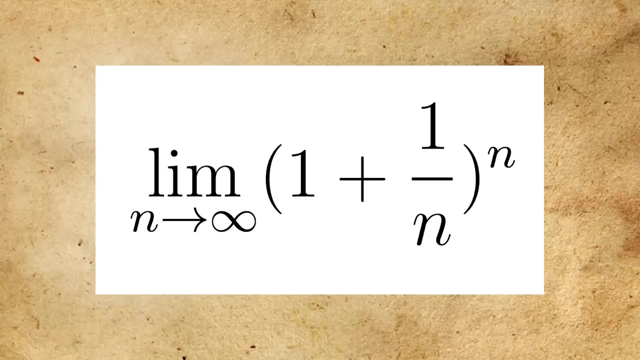 It's a constant 2.7 blah blah blah. named by Leonhard Euler, Of course named after him, But it is essentially an infinitesimal over 1, multiplied by itself infinitely many times, or defined like this or this: 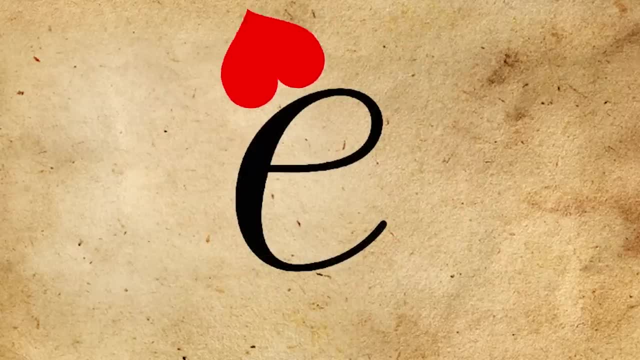 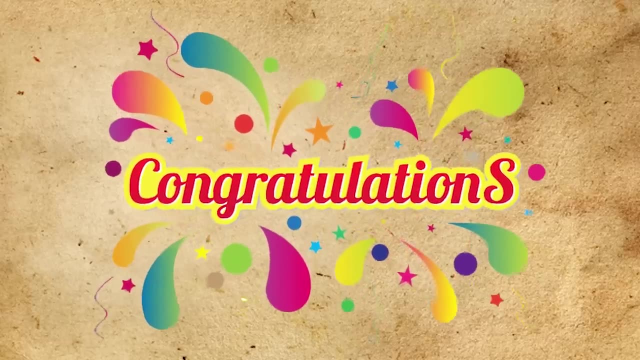 And mathematicians love it because it's very natural and shows up literally everywhere. in math It's like a cat that always shows up when you least expect it. Congratulations, We made it through all the realistic numbers you'll actually use. Of course, there are more. 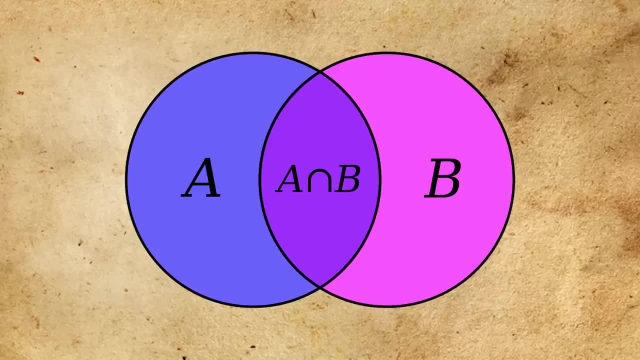 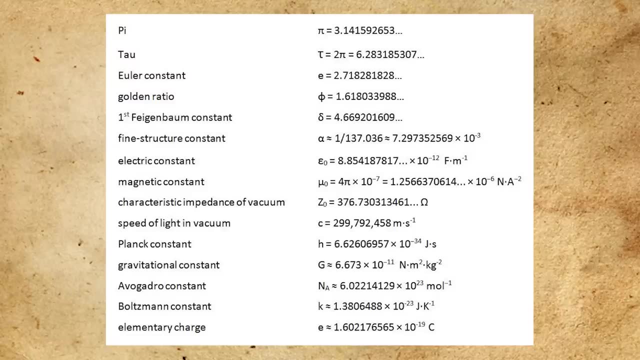 It's math, after all. You can sort them. you can make your own sorters. put numbers in a square, count infinities, go hypercomplex, go p-adic, or, of course, there's a whole world of important constants. 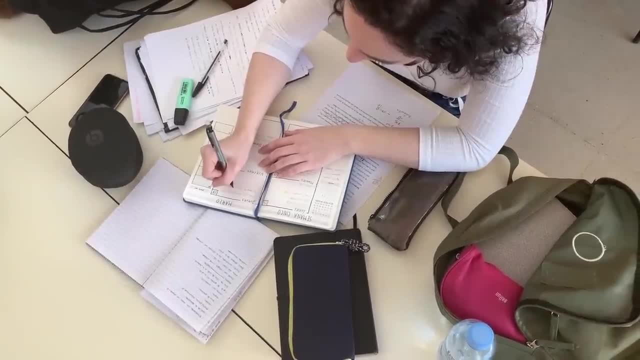 in numbers. Why don't you study hard for a PhD in mathematics? I'll see you next time. Bye, Bye.